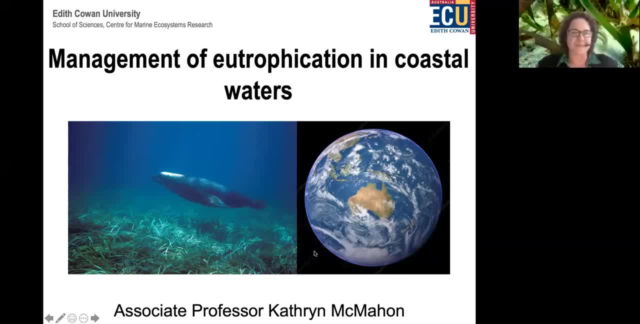 Hi everyone. Thanks so much for inviting me along today. I'm really excited to chat to you and share a bit about myself. My name is Catherine McMahon, I'm an associate professor at Edith Cowan University and I'll be talking to you today about management of eutrophication in coastal 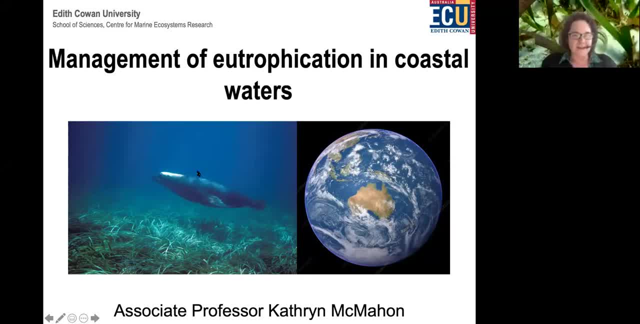 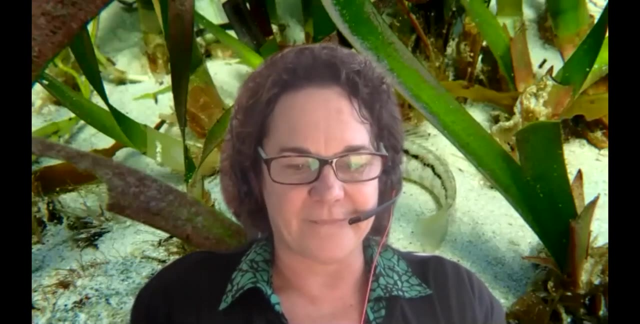 waters. Okay, I'm just trying to move to the next slide. It seems to be stuck. Yeah, it's stuck, so I'm just going to go out and stop sharing and then I'll try again. Don't worry, we can clip this bit out. 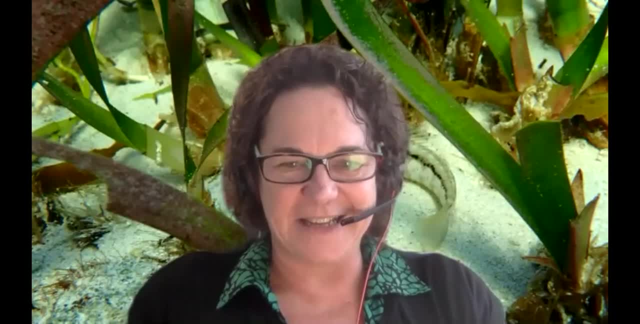 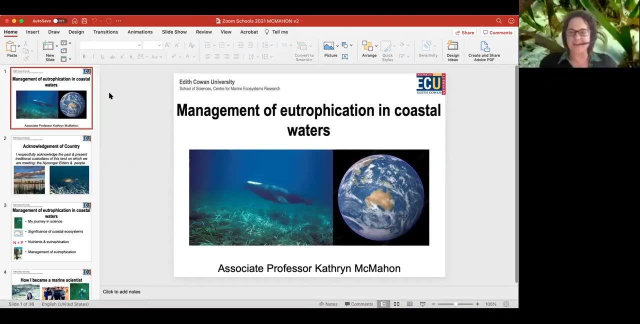 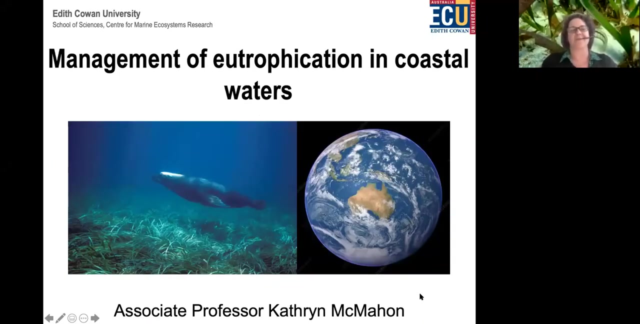 Great, So you can see those slides. I'm just going to go into presentation mode and double check that it's going to move through. It is going to move through now. Okay, so this is the official start. So I'm going to talk to you today about the 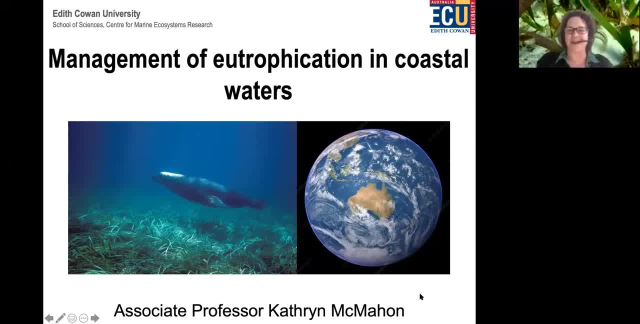 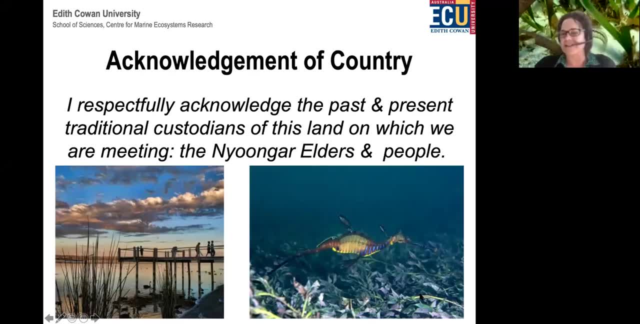 management of eutrophication in coastal waters. Thank you for having me along The first start. I'd just really like to acknowledge the traditional owners, the Noongar elders and the emerging and past and present whose land in which we're meeting today, because we all are in Perth. 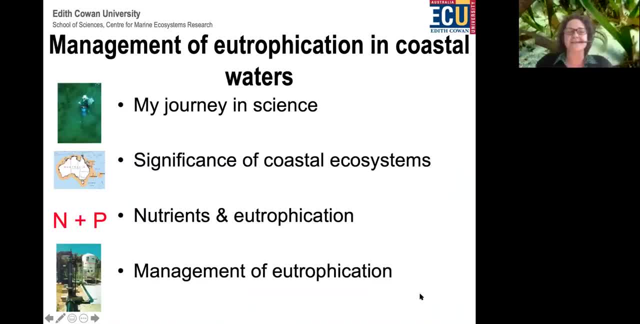 And so what I'm going to do today is talk to you about four things in this presentation: A little bit about my journey in science and how I got to where I am today. The significance of coastal ecosystems. The significance of coastal ecosystems. The significance of coastal ecosystems. 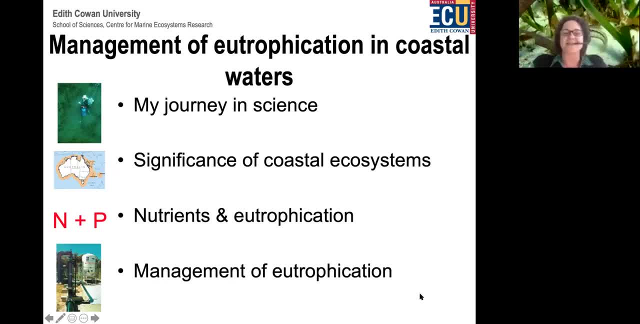 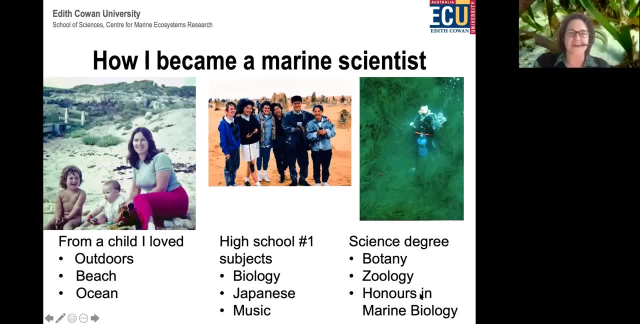 Benefits of łores wheel or eutrophication, And then specifically on nutrients and eutrophication And some of the management approaches that we can use for eutrophication. So from a child I just loved the outdoors, the beach and the ocean. I grew up on the beach. actually, I grew up very close to your school in. 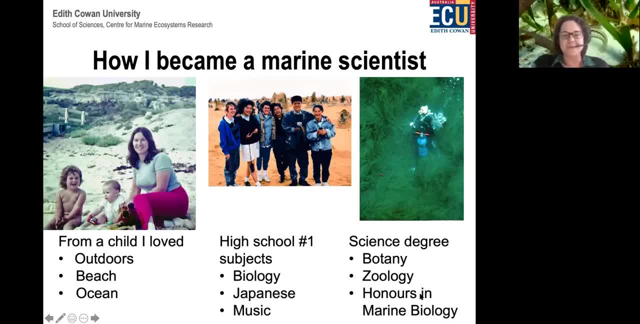 Mullaloo, and then I went on to high school and I was really interested in Japanese and music, um, and so I went to Greenwood Senior High School and that's all right, because I could do both Japanese and music there, but when I was at high school I just really loved the subject biology. 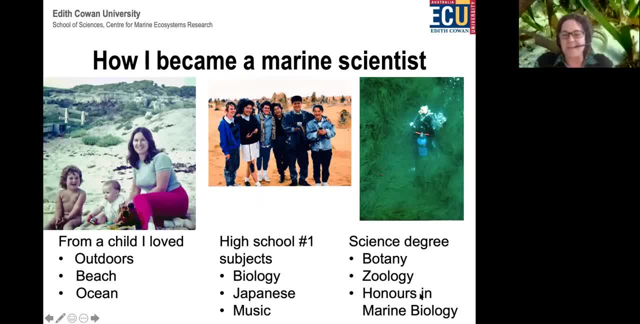 and it was that love of biology that made me want to go to university, where I did a science degree and I studied botany, plants and zoology animals, and then in my final year I did a. it's an honours program, so it's a special one year where you do a research project and that's actually me. 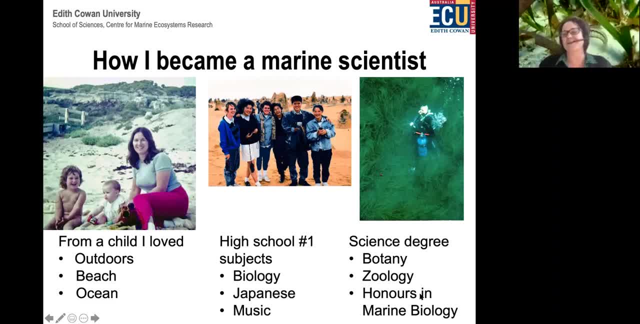 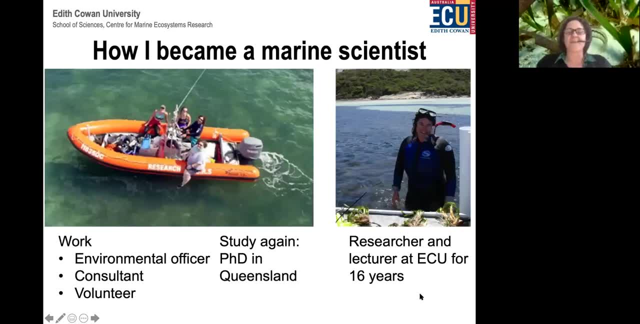 in 1994 in Geograph Bay scuba diving doing my my honours project on the right hand side of the screen. When I finished university, I did a variety of different jobs. I worked as a consultant and I also worked as an environmental officer, and that was where I really started my journey into water. 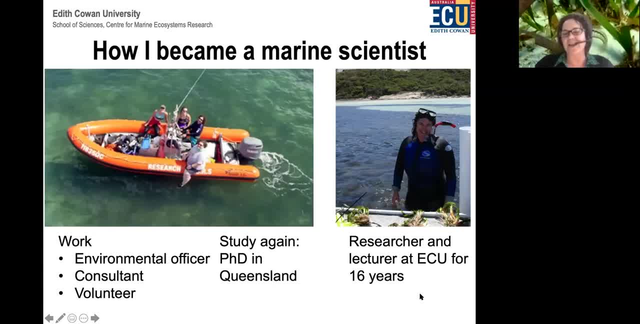 quality and I started to start to spend two years working for the. at the time it was called the water and rivers commission, but now it's the department of water and environmental regulation and I worked with them. I went out on a boat once a week measuring water quality in the Swan River estuary, so that was a really 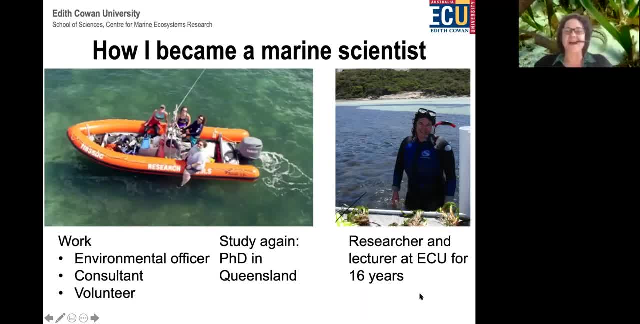 a really great job, but in the back of my mind I always just really loved doing research. so I went back to university again and did something called a PhD, where you study for three to four years on a particular research topic, and I did that in Queensland. that's me driving the boat on the left hand side of the screen and my study was on dugongs. 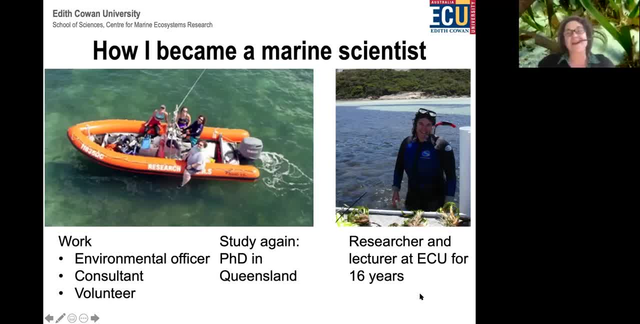 and seagrasses, which was really exciting. then, when I finished that, I moved back to Western Australia and I got a job at Edith Cowan University and I've been working there for about 16 years doing research particularly in coastal ecosystems and seagrasses. 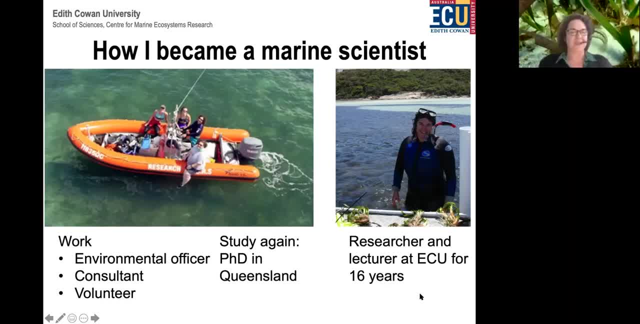 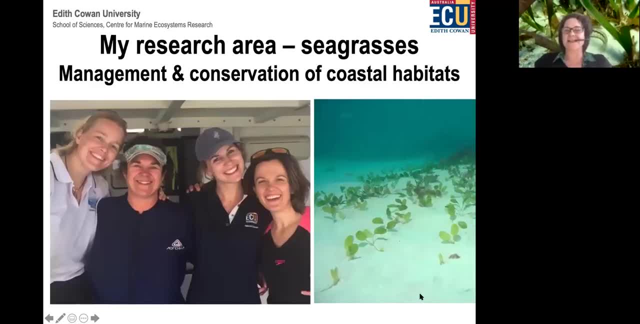 and also teaching in environmental science. so that's my story about marine science, and the area that I work in is in the management and conservation of coastal habitats. so I work with people from government agencies, from industry and a range of students doing studies to improve the way that we manage and conserve coastal ecosystems. so why do we care? 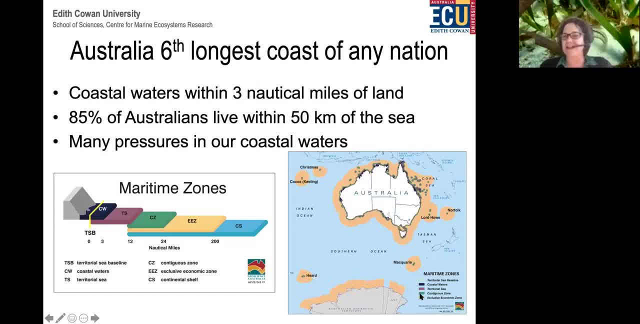 about coastal ecosystems. well, Australia is quite unique in that it has the sixth longest coast of any nation in the world and these coastal waters, they're essentially from the land to about three nautical miles out into the sea, and 85 percent of Australians live on the coast, within 50 kilometers of the sea. so because 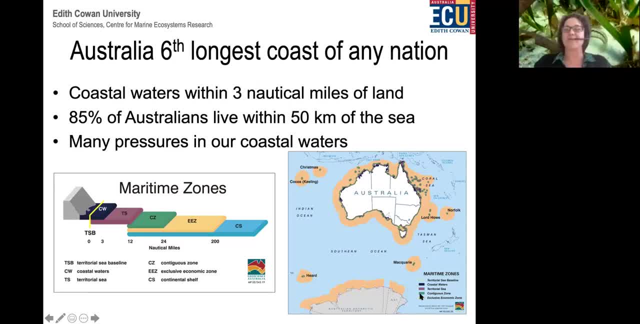 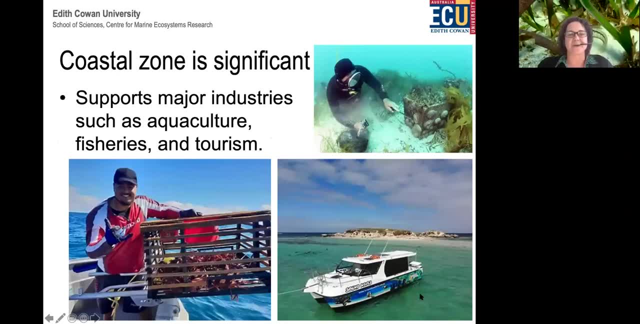 most of our population lives there. there's actually quite a lot of pressures in our coastal waters now. it is a really significant zone. it supports many industries, so there's aquaculture. so in the picture on the top right is actually the Abaloney Farm down off Augusta. we have really important fisheries in. 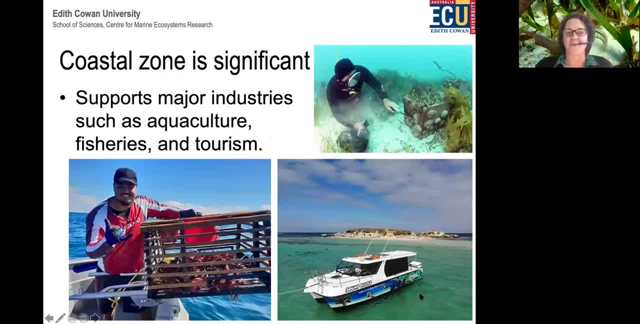 our coastal waters and I'm sure many of you are aware of the rock lobster industry, tourism, shipping. most of the things that we buy that come from overseas get into our shops through shipping. so the ocean is a really important conjuction. do it for our economy. Now the coastal zone. they're highly productive. So if you have a look, 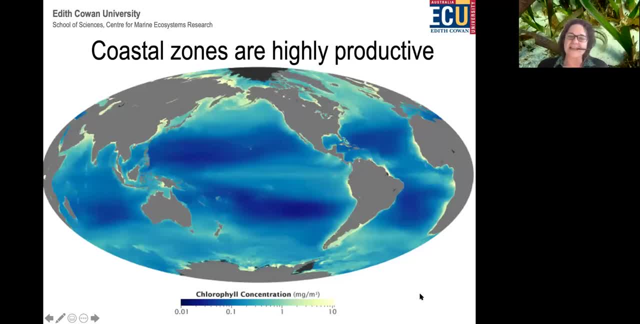 at this map of the globe. the colours of the water are showing you the concentration of chlorophyll. So chlorophyll is a pigment. It's a pigment that is found in those tiny cells that photosynthesise the plankton, And when these plankton photosynthesise, they use sunlight and 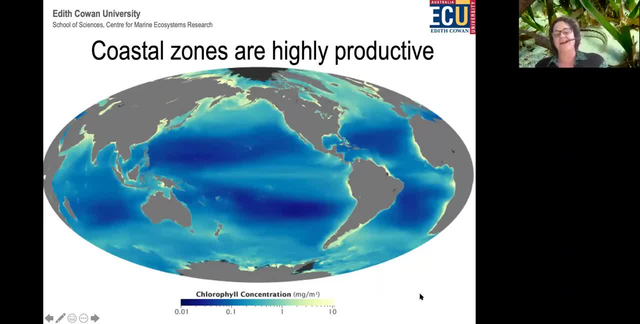 carbon dioxide to produce oxygen and organic compounds which form the basis of many food webs. So you can see where the yellow is. that's a higher concentration of chlorophyll, meaning a higher concentration of phytoplankton and more productivity. And these yellow 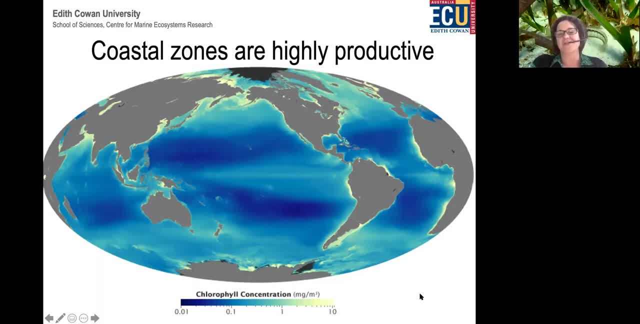 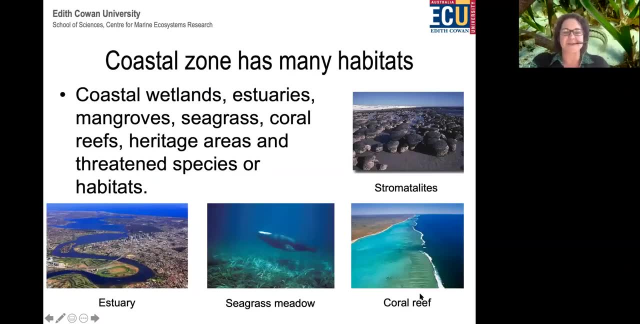 colouring is always around the edge of the continent. so in the coastal zones Now there's lots of different habitats in the coastal zones as well. So we have wetlands, estuaries. so the picture on the left you can see. I'm just going to move around because the sun's shining on my computer and I can't see it. 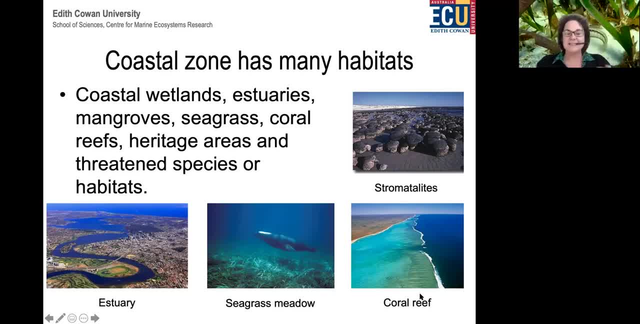 There's the estuary, the Swan River estuary, on the left hand side, Seagrasses- that picture in the middle form really important habitats. We have coral reefs up in the middle, up in Ningaloo, And in that top picture is stromatolites, which is in Shark Bay in the World Heritage Area. 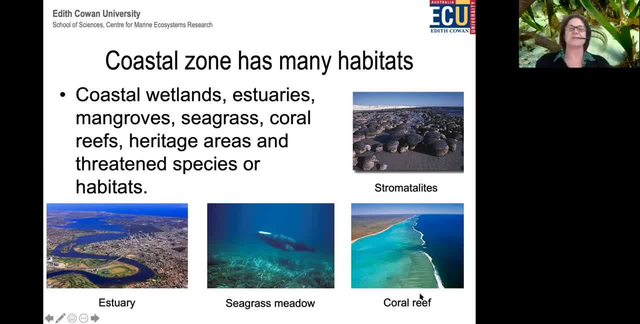 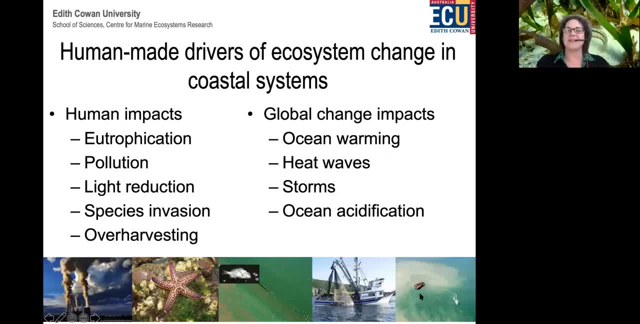 So many threatened species and habitats live in this coastal zone. Now, as you're probably aware, there's many human activities that are impacting the coastal ecosystem and driving ecosystem change- Things like global warming, ocean warming, heat waves, storms, ocean acidification- But what I'm going to talk about today is some of the human impacts that occur more at the local scale, and that is eutrophication. 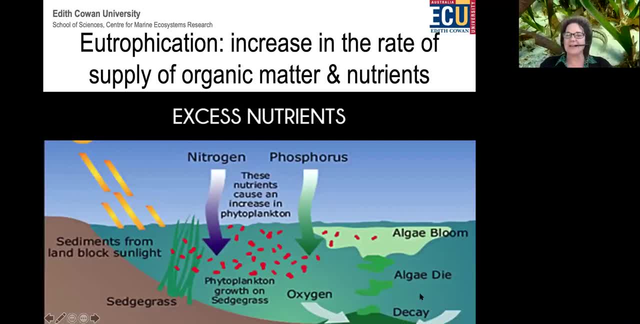 So eutrophication is an increase in the rate of supply, so the amount of both organic matter and nutrients that move into our coastal waters or any aquatic ecosystems. So if you look at that picture on the bottom, you have organic matter or nutrients like nitrogen and phosphorus coming into the system. 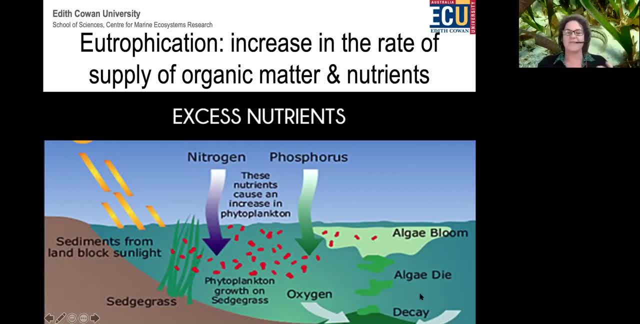 Now, when these nutrients are being added at a faster rate, it causes the phytoplankton and the algae to grow really rapidly and create these blooms. And then, when these phytoplankton and algae bloom, that just means there's lots of cells there. 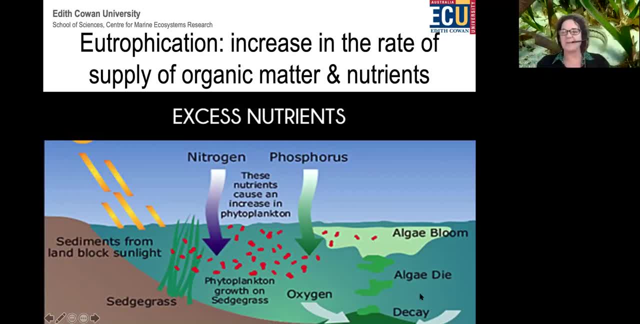 eventually they die. They drop down to the bottom of the water column, They sit on the seabed. That's what we call sediment And there's a lot of organic matter, so dead cells, essentially. And whenever there's something dead, you get bacteria or fungi that break that down and release the nutrients back into the system. 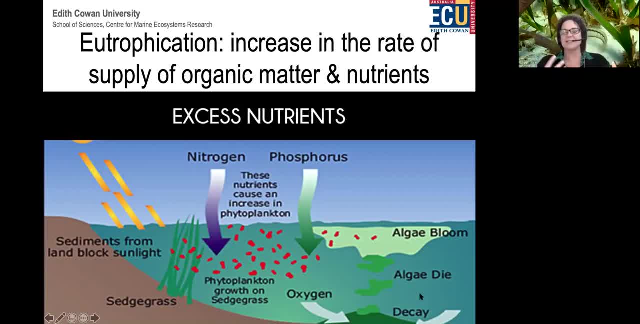 So the bacteria and the fungi. they need oxygen to survive, because all organisms use oxygen for respiration, or the majority of them. So when they're in the water body consuming all this material that's breaking down, then the oxygen is going to be in the bottom of the water column. 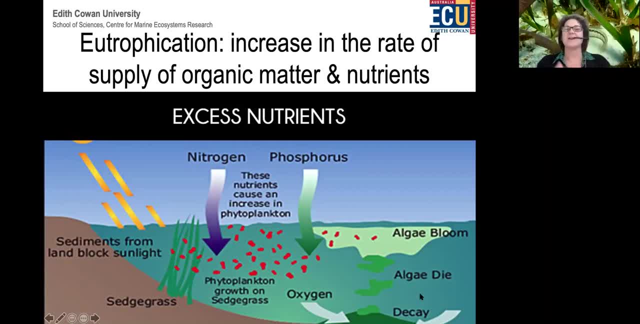 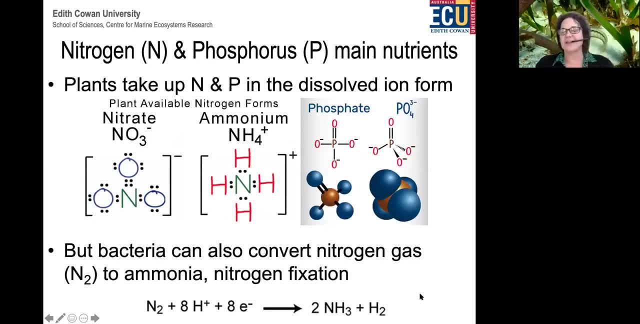 So when they're in the water body consuming all this material that's breaking down, then the oxygen is going to be in the bottom of the water column. concentrations in the water body come down. so this is the process of eutrophication. now the key nutrients that drive this process are nitrogen and phosphorus. so nitrogen and phosphorus. 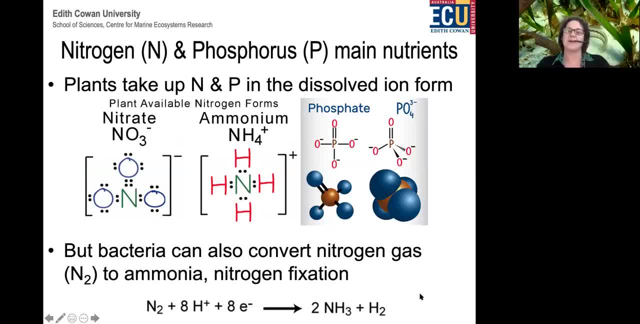 can be, can be delivered to the aquatic ecosystems, either as particles or organic material, bits of broken up leaves or small dead animals, or they can also be in the dissolved form, so as ions dissolved in the water, and when it's, the most common forms are nitrate, so we have nitrate on. 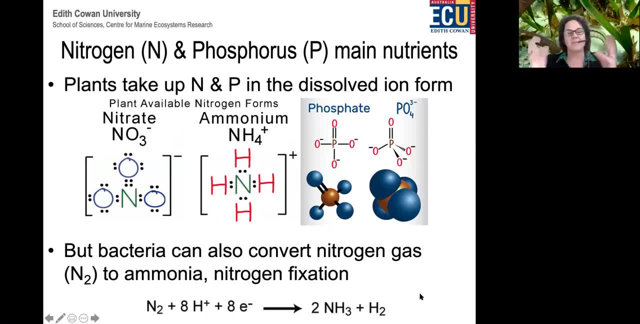 the left of the screen, which is one nitrogen atom bound to three oxygen atoms and it has a negative charge. ammonium is another important form of nutrient. so that's one nitrogen atom bound to four hydrogen atoms and it has a positive charge. and then phosphate, another way that nutrients can come into the. 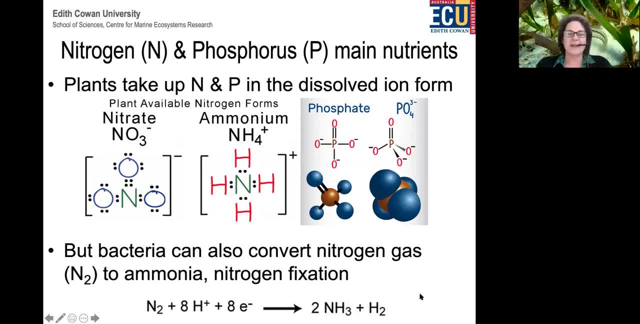 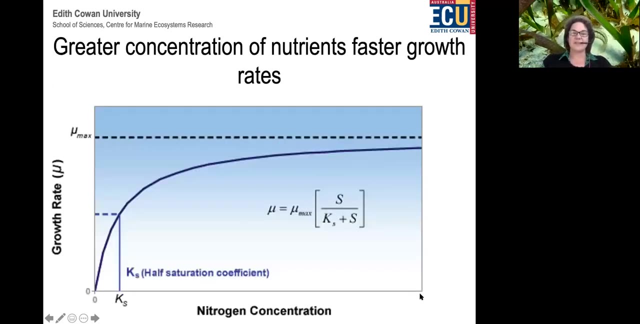 system is by bacteria, so bacteria can use actually nitrogen gas and they can convert that nitrogen gas to ammonia, and when it's dissolved in the water, that becomes ammonium, and so that's another way that organisms can access nutrients in in aquatic environments. you now, what this graph is showing is that as the concentration of nutrients increase in the water, 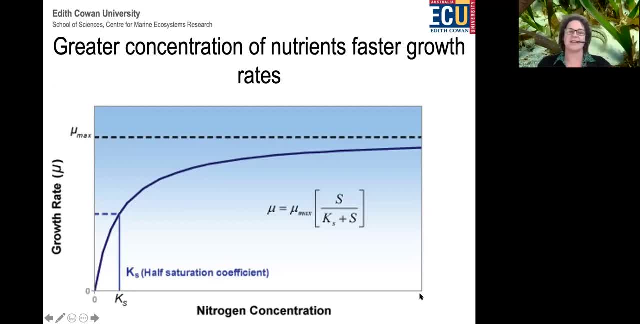 body because there's an increasing supply under eutrophication that will increase the growth rate. so if you look on the x-axis, the bottom axis of that graph, where on the left hand side is zero or a low concentration of nitrogen, and as you move along the axis towards the right, that concentration 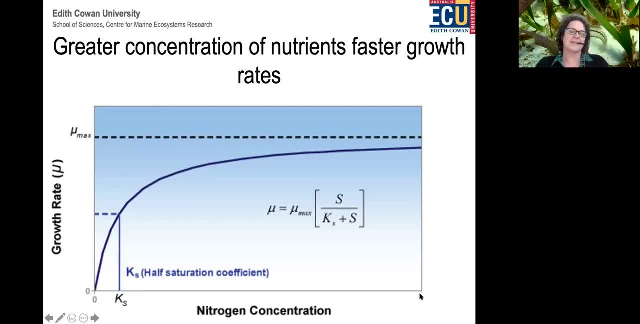 is increasing and as you move along the axis towards the right, that concentration is increasing. and you can see on the y-axis that initially there's a rapid increase in growth rate and then it starts to peter off and as the nutrient concentration gets higher it sort of reaches the slope and you're not going to get any faster growth. 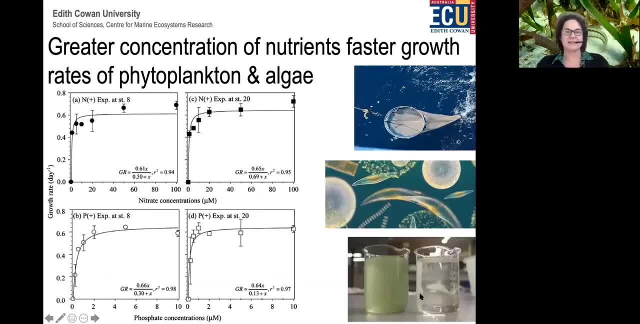 so that's conceptually what you'd expect, and what we have here are some graphs of the growth rates of phytoplankton collected from oceanic waters or coastal waters. sorry, so that net that is in the top picture on the right hand side of the screen. 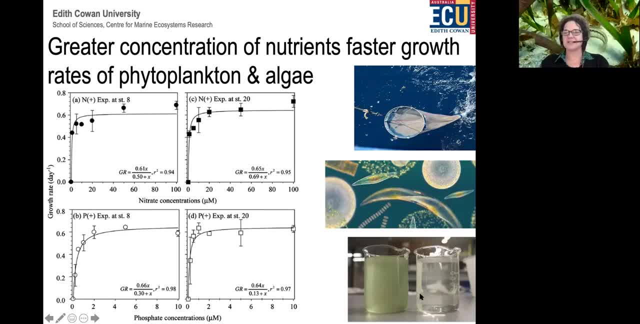 essentially it's dropped into the surface waters. you drag the net along and there's a little tube at the bottom of the net that filters. the water comes out and all the phytoplankton collects in that tube. so the middle picture is just showing you some different cells that are phytoplankton. 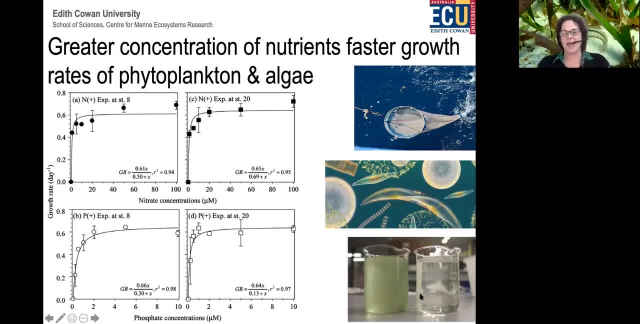 and then, in a simple experiment, you add those cells with some of the phytoplankton and you get a little tube that filters the water out of the sea water into beakers or into jars, and then you have multiple jars with different concentrations of nutrients and then you measure how the number of cells in that jar increases over time, and that's. 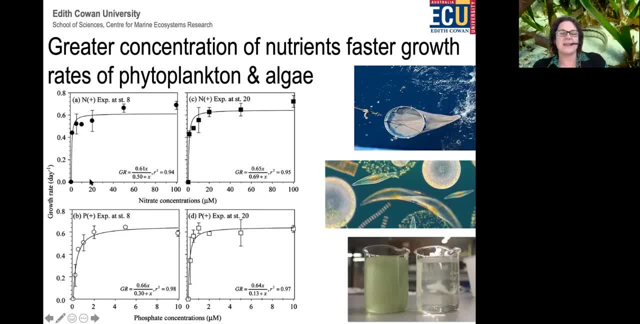 how you work out the growth rates. so in the graphs that you can see on the left hand side, the top one is when nitrate has been added and the bottom one is where phosphate has been added. so you can see, from zero up to about 10, this rapid increase in the growth rate of those plankton, with increasing. 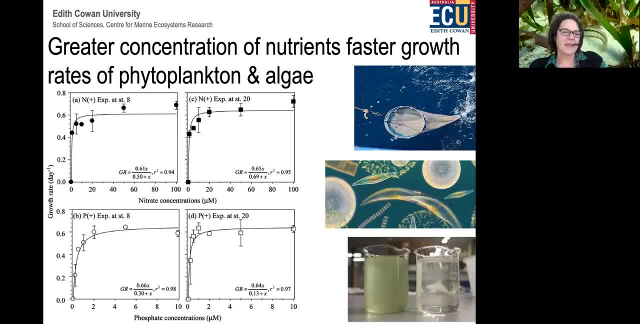 nutrient concentrations and interestingly, if you look at the nitrate it sort of reaches the maximum kind of growth rate at around 20. if you're looking on the x-axis you go from zero to 20 and then if you go up the graph you can see the growth rate is around 0.6 per day and then if you go up the 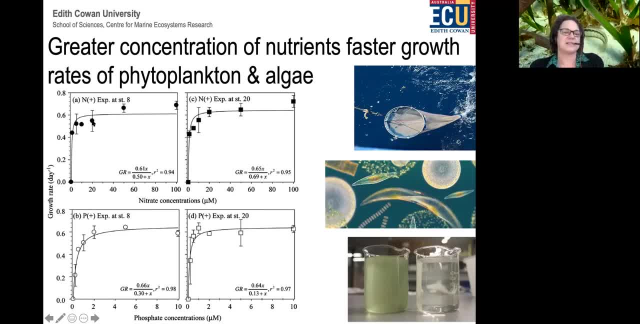 x-axis, you can see the growth rate is around 0.6 per day. that's where the growth rate saturates at 20 micromolar concentration of nitrate. but it happens at a lot lower concentration for phosphate, so at around 2 micromolar for phosphate. that's where you see that the curve of the graph flatten off. 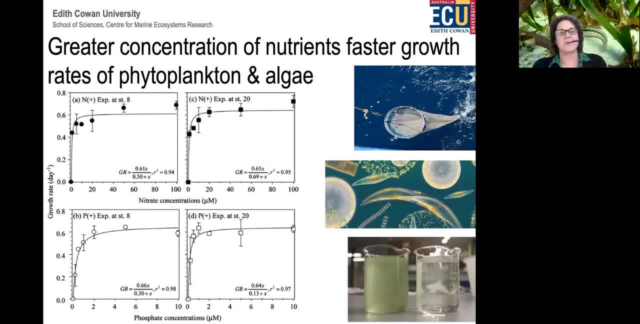 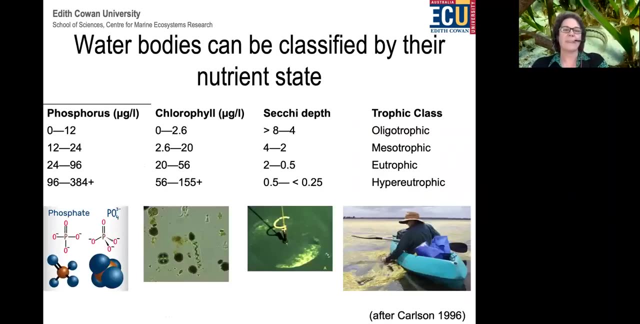 so plants. most plants require a much higher concentration of nitrate nitrogen than they do phosphorus. so it's not just that total amount but also the ratio of the nutrients that can affect the growth rates. so water bodies can be classified by their, their nutrient state and some of the factors that are. 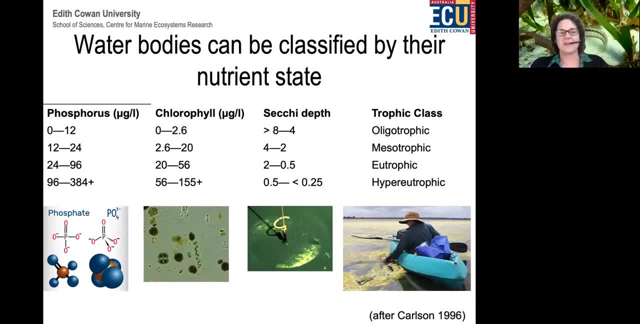 included in this kind of classification are the concentrations of nutrients like phosphorus, which we have on the left hand side, and on the right hand side you can see that the states are oligosaccharides, which is the lowest concentration of nutrients, that usually have the lowest amount of chlorophyll in. 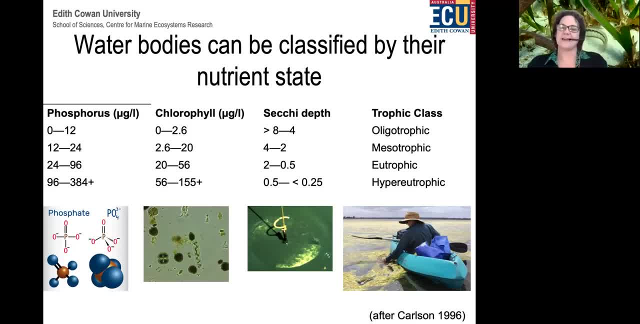 them and higher secchi depth. so a secchi depth is a scientific instrument. it's a really basic one and you can see it in the picture. it's sort of a rope with a round disc and the disc is divided into quarters. two quarters are black and two 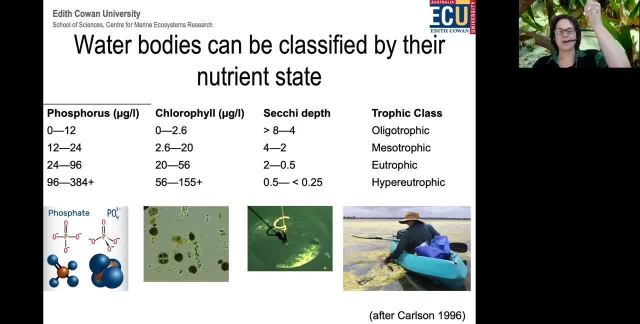 quarters are yellow and two quarters are black, and two quarters are black and two quarters are white in color. so you lower that disc down and when you can no longer see the difference between the black and the white quadrants, that's called the, the secchi disc depth. so the deeper or the 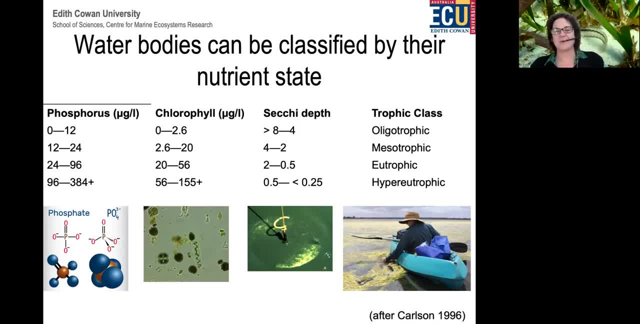 higher the secchi disc depth, the clearer the water is, and the lower the secchi disc depth, the more phytoplankton and more turbid the water is, so it's much harder to see. so as you go from egotrophic to mesotrophic, to eutrophic. 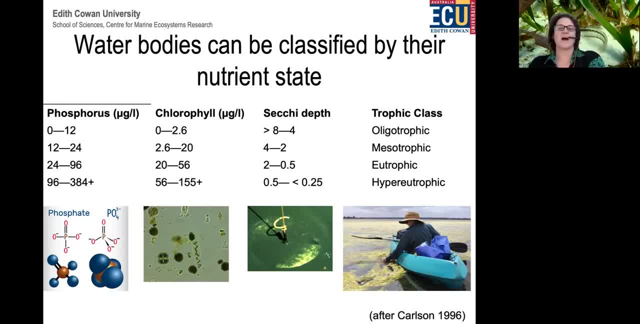 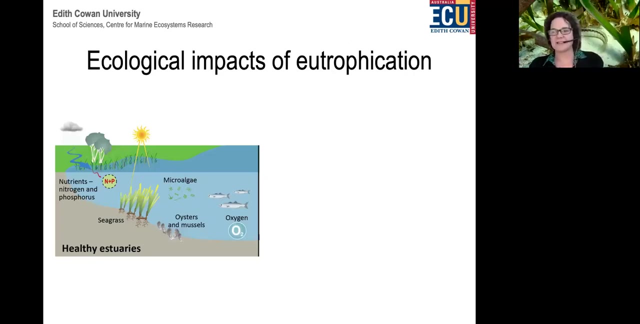 this is sort of. if this is just in one location, you'd be seeing the process of eutrophication: increasing nutrients, high concentrations of chlorophyll in the water and less clarity in the water because there's so much phytoplankton. so when eutrophication occurs, you get a range of changes in the ecosystem and i've talked about a 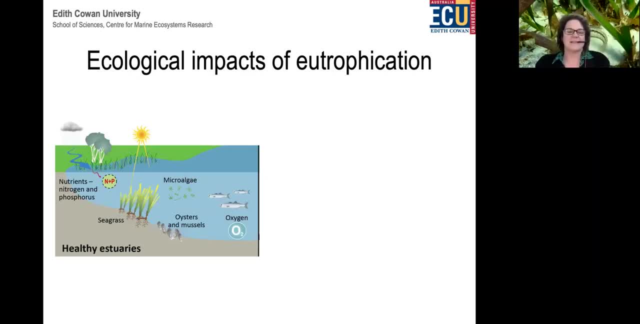 few of them in the past, but i'm going to talk about a few of them in the next few minutes. so if we just think about and, as an example, estuaries and think of this as the the swan river estuary, if you like, so there's nutrients, nitrogen and phosphorus that come into the estuary through. 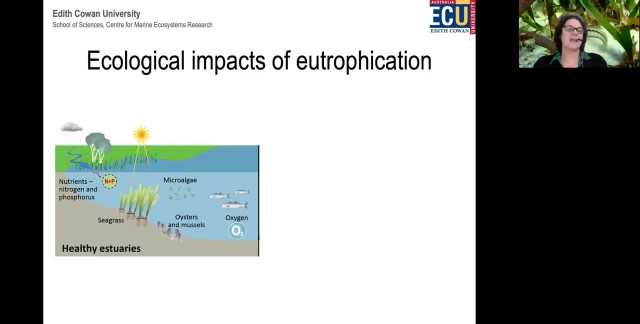 a variety of catchment activities and then those nutrients are used by the phytoplankton or microalgae to grow. they're used by the, the seagrasses, the plants that grow on the bottom, the microalgae and the seagrass and the phytoplankton and the phytoplankton and the phytoplankton and the. 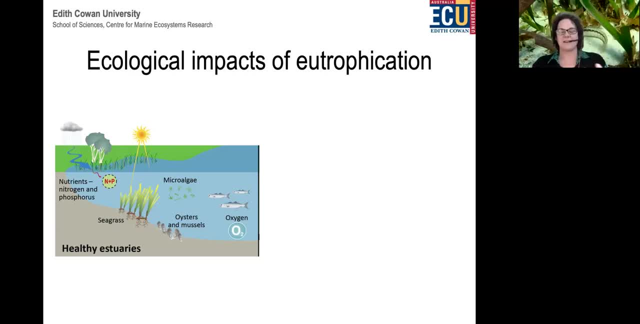 seagrasses produce oxygen and it makes it a healthy environment for fish and other organisms to live in. now, when you have eutrophication, you have increased loads, increased amounts of nitrogen and phosphorus coming into the system from a range of activities in the catchment. those 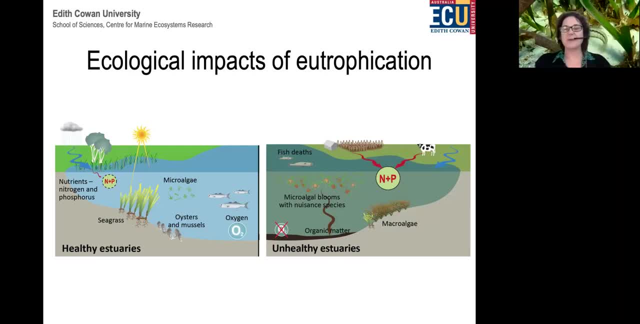 concentrations stimulate phytoplankton blooms, but not only phytoplankton blooms. also, if you look on the right hand side of the picture, macroalgae, so fast-growing, filamentous or different types of macroalgae that tend to grow over the seagrasses and kill the seagrasses. so this high. 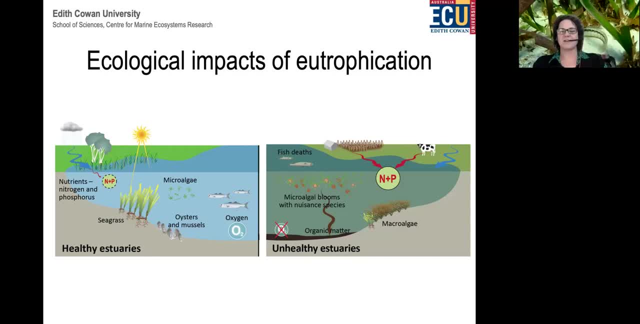 primary production. then when, when it dies off, it drops down to the bottom of the estuary where you get this big build-up of organic matter. drawing the and the breakdown of that organic matter reduces the oxygen concentrations. if there's not enough oxygen in the water, then the organisms that 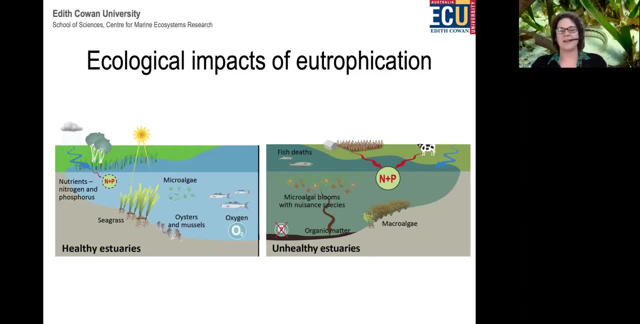 are living there are going to die, like fish or any the oysters and mussels that are living in or on the sediments. so this is sort of like the, the ecological change that can occur when eutrophication happens. and another interesting thing: it's not just the total. 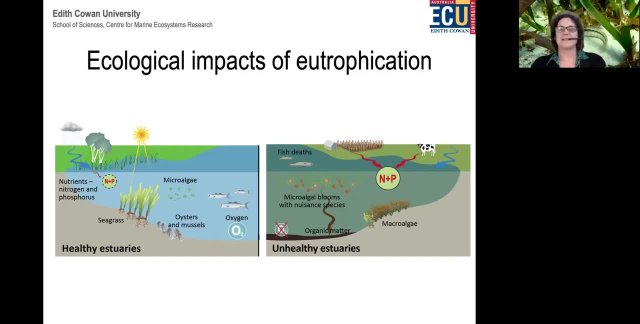 amount of microalgae or phytoplankton that increases. it's also the type of microalgae or phytoplankton that change, and often under eutrophication, you it's more common to have species of phytoplankton that are actually toxic, so they can cause impacts to other organisms that 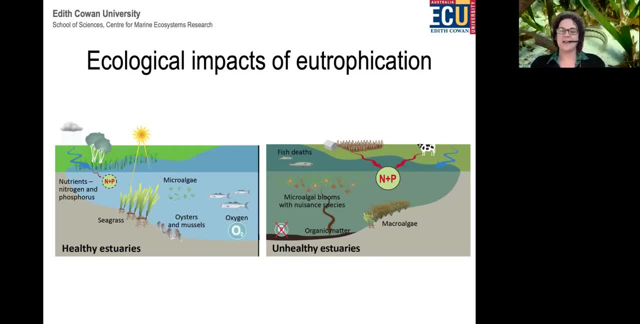 either feed on them or are exposed to the water. so some of these toxic algae and phytoplankton that are actually toxic algae can form like these toxic compounds that are called, like paralytic, that cause paralytic shellfish poisoning that not only kills or impacts the organisms, but if we eat them. 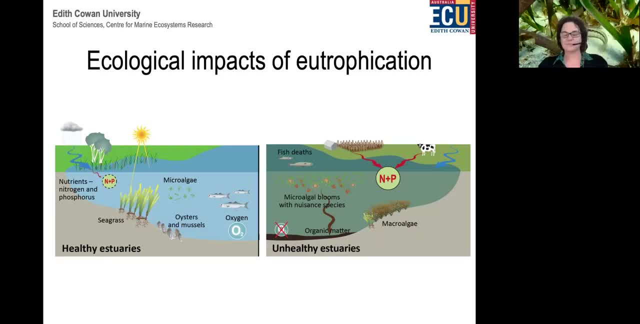 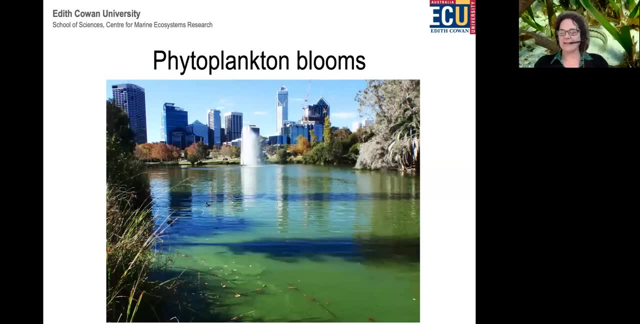 as humans, we can also be impacted, so eutrophication is actually really common around the world, and we see it in the southwest of western australia, where we all live. this is an example of a phytoplankton bloom in a lake around the the swan river, and you can see all those green like. 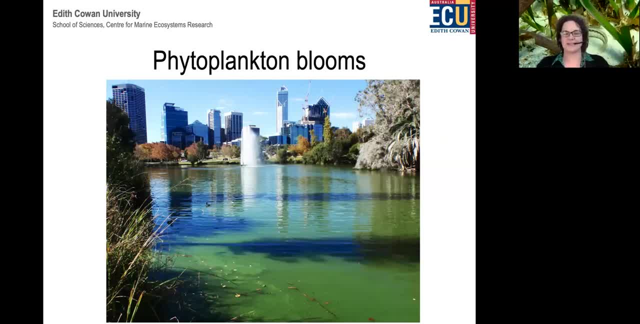 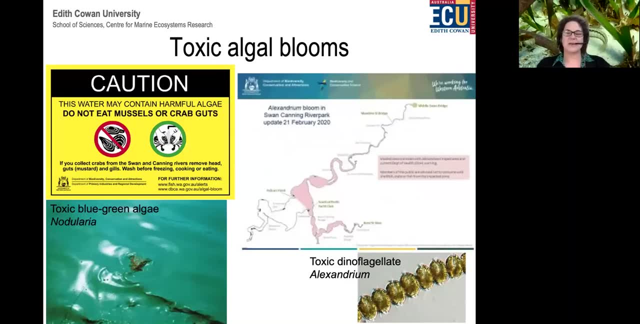 the water is a green color that's full of phytoplankton in the water. this is an example of a toxic algal bloom. so on the right hand side you can see a map of the swan river where it is red. this is where the toxic algal bloom. 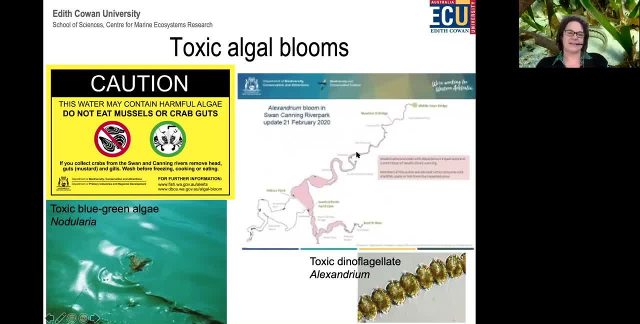 was present and where it was recommended that you couldn't eat the mussels or you needed to clean the crabs before eating them because of this toxic algal bloom. and it's actually. this is a. on the bottom right hand side you can see the picture. it just looks like a. 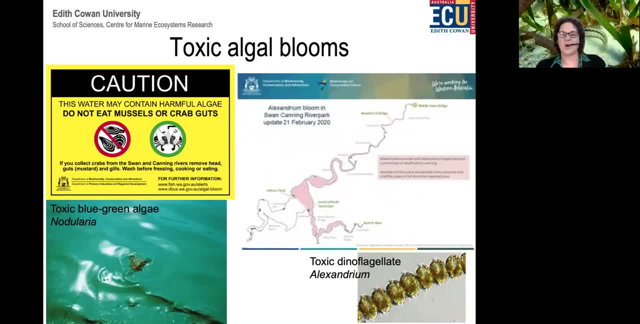 a chain of i don't know six golden brown cells. these are the cells that grow really quickly and they form these chains. they just all join together and each individual cell has that toxic toxin in it that causes this. shellfish poisoning on the left hand side is another type of toxic algae. 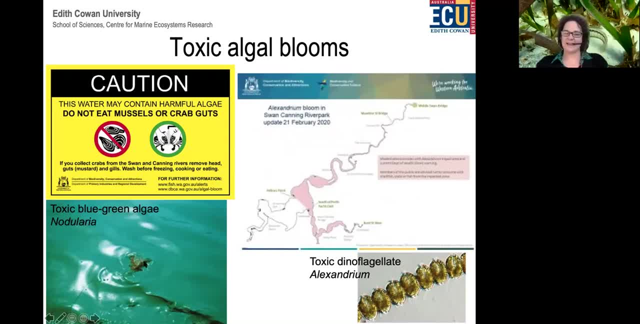 called nodularia and it just looks like someone has poured green paint into the water, and these have been quite common in some places in southwest western australia and they impact fish. and also, if you get your skin exposed to that, if you walk through that water, your skin would get really itchy as well. 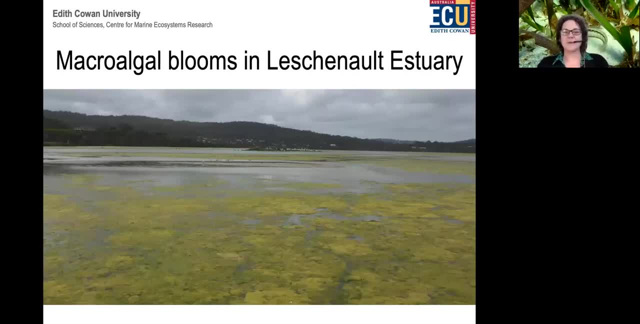 this is an example of a macro algal bloom. this is the leshinal estuary, which is down near bustleton. some of you may have gone crabbing there at some stage. it certainly was something i did quite regularly as a kid, and in this case it's a very, really shallow water body. 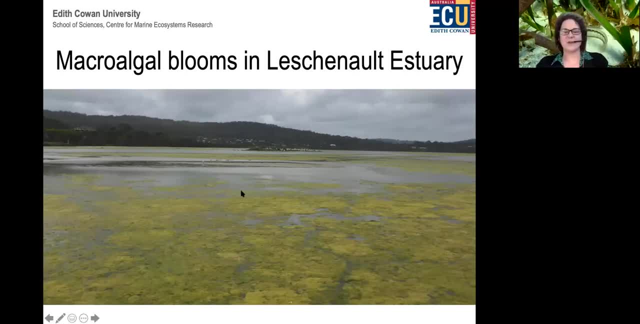 that has all this sedimentary algae and all these fillamentous algae outside. it is just a lot of nutrients, of nutrients coming into it, and these, what you can see floating on the surface of the water, is all this filamentous algae that grows really quickly and just forms a matte over. 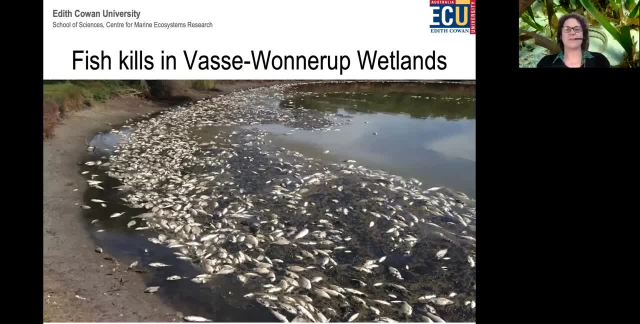 everything, and i'm not sure if you've heard, but there's been quite a number of fish kills in the vaswannaup wetlands, and this is a wetland of international significance near bustleton, and what happens here is that we don't only see here, but we see a lot of fish in the environment. 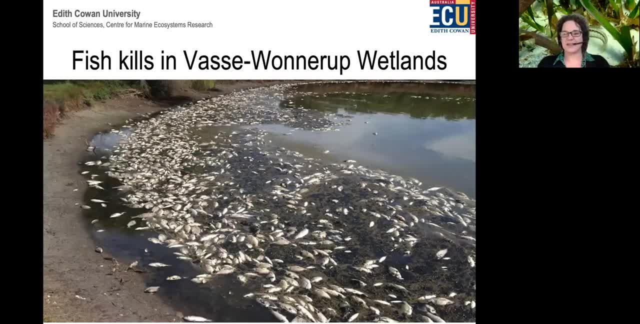 so this is something that we don't really get to see in the clean water, and that's really bad, really bad. it's a highly eutrophic system, and either there's toxic algae or, in this case, the oxygen concentrations were so low and the fish couldn't escape that there was a big die off of fish. 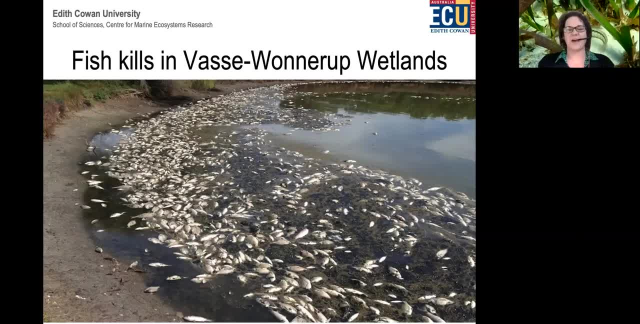 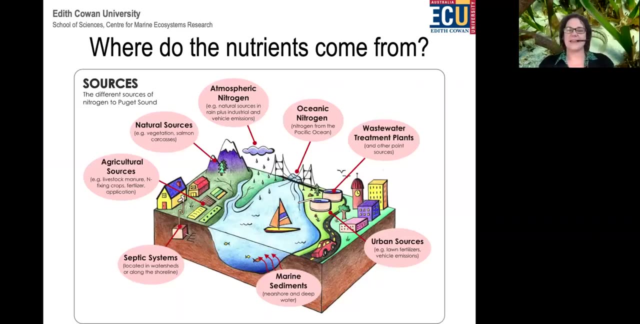 and actually this. this photo was from about four years ago, but actually a big event happened just last week and I think about 20,000 fish died. So clearly, if our waterways are getting increasing supply of nutrient, there can be these catastrophic impacts, and these nutrients can come from a range of sources and they can actually 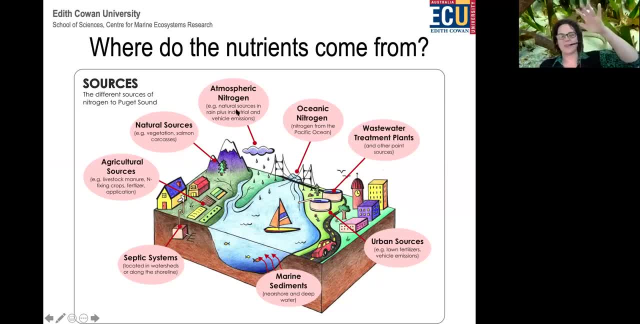 come from the atmosphere, so just falling with rainfall, and it is mostly due the nitrogen in the rainfall. It's mostly coming from the burning of fossil fuels and, like vehicle emissions, that can have high amounts of nitrous oxide in them, so they get. when the fossil fuels get burnt, the the gases go. 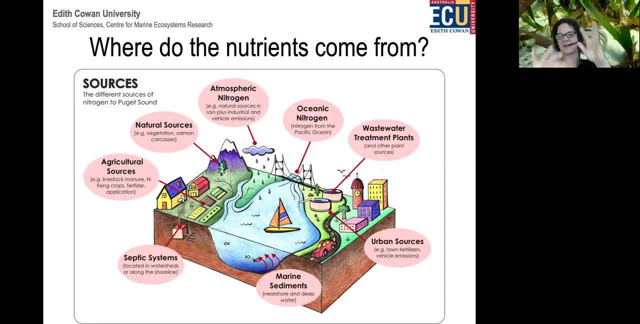 into the air and they join with the particles of the rain and get rained down as dissolved nitrate. Wastewater treatment plants are another big source of nutrients. so anything, essentially anything that's going to be used to make a good nutrient is going to be used to make a good nutrient. 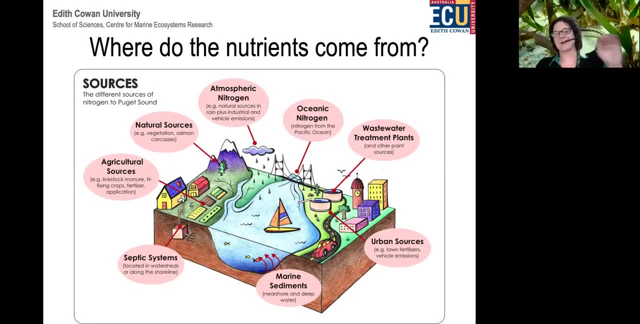 So anything, essentially anything that's going to be used to make a good nutrient, is going to be used to make a good nutrient. So anything that goes down our toilet or down our sinks and goes to the wastewater treatment plants. they get processed and a lot of the nutrients get removed and then they most usually get. 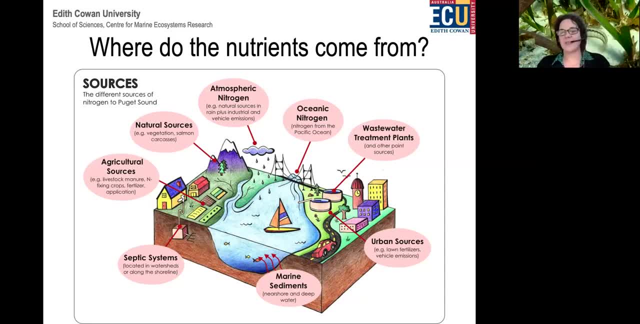 discharged into the marine environment. Nowadays there are some places where they get discharged into the groundwater, So wastewater treatment plants are a big source of nutrients, Just our urban environments. if we have gardens, or also vehicle emissions that I've already mentioned, you fertilize your garden and the nutrients drain. 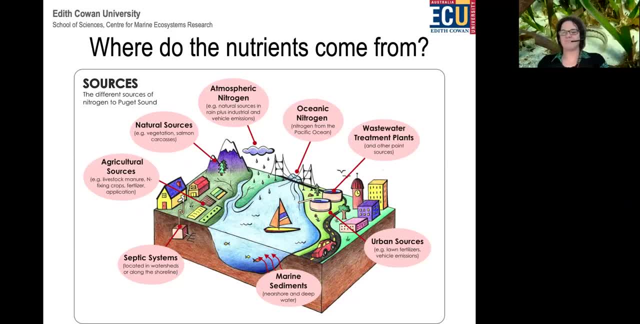 into the groundwater or into the, the stormwater drains, and then they get washed into our aquatic ecosystems. Agricultural sources. so if you have you're growing wheat or barley or vegetables, or if you have livestock, there's usually a range of either nutrients that you add to help your crops grow or the manure from the livestock that you have. 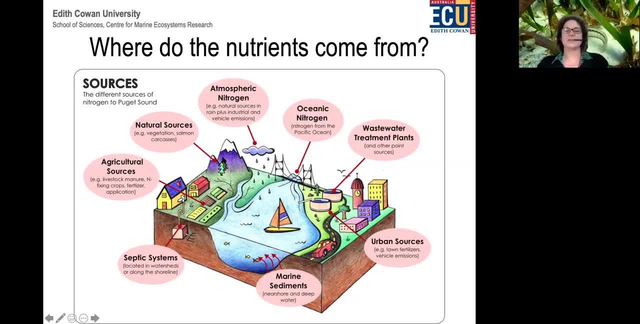 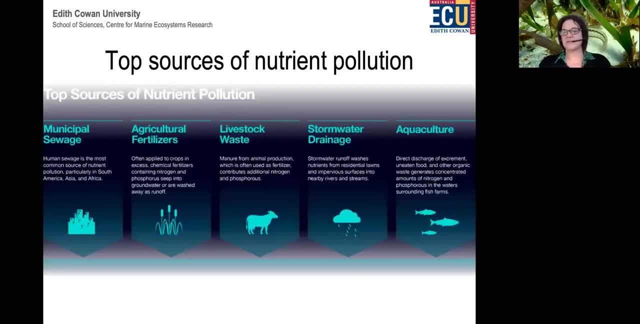 can leach into the waterways and increase nutrients. So a whole range of sources, But the top sort of sources of nutrient pollution that reach our aquatic ecosystems usually come from the wastewater treatment or sewerage, the agricultural fertilizers, livestock waste, our stormwater drains and also aquaculture. 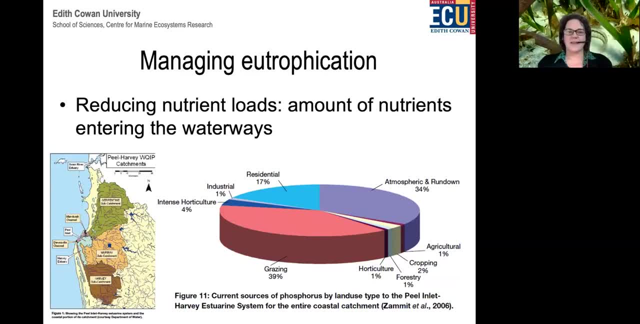 So what I want to move on to now is just talking about: okay, so we know that this is happening in our aquatic ecosystems, in our coastal systems, which provide these really important ecological services for us. So what can we do to actually manage eutrophication? 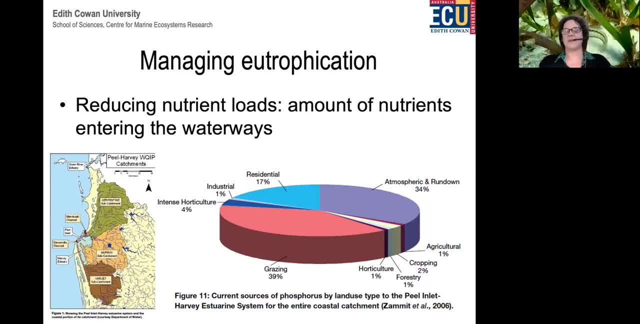 And this is something that many people have been working on for decades, because eutrophication is not an emerging issue. It's been around for a long time And usually a lot of government agencies manage eutrophication, So a key way to do it is to manage the loads. 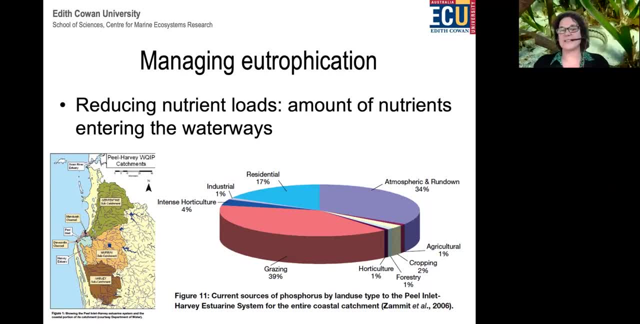 So the loads are the total amount of nutrients that are going into the waterways. So this is an example where people have monitored all the drainage, all the rivers and drainage systems that are going into the Peel Harvey Estuary. So this is down in Mandurah, just south of Perth. 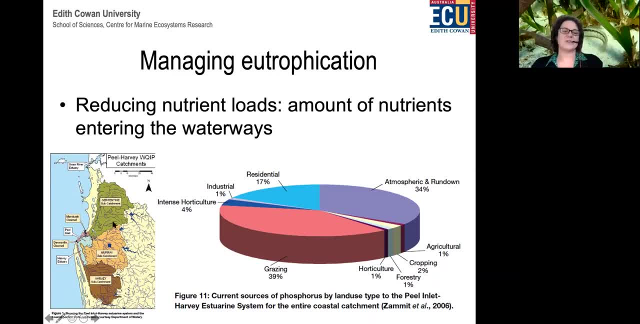 You can see that there's a range of catchments. So there's the serpentine catchment, the Murray catchment, the Harvey catchment, and they all have rivers and drainage systems. You can see them, the little blue lines on the map. 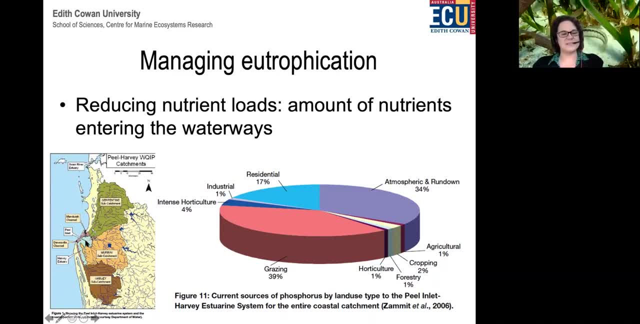 that when they fall, the water flows into the Peel Harvey Estuary, that little blue shape on the left hand side of the graph. they're made up of the Peel Inlet and the Harvey Estuary, So they work out the amount of nutrients coming in from all. 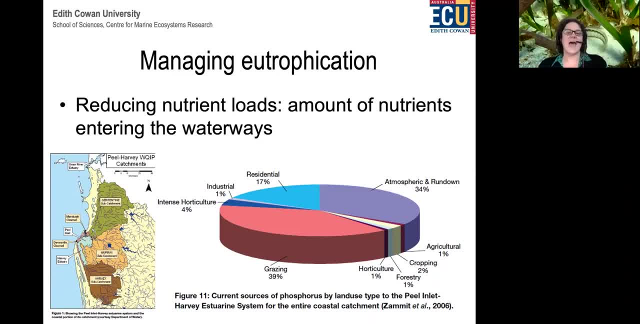 these different tributaries, these little rivers, and the type of land use that's occurring in those tributaries, And then they can work out the proportion for each sort of land use activity where the nutrients are coming from. So if we look at this pie chart in the bottom right of the graph, 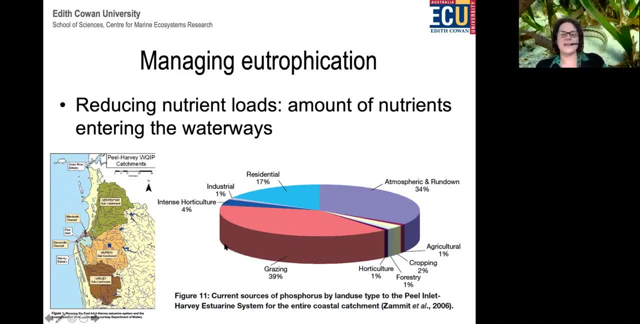 of the page- sorry. you can see that the greatest proportion of- in this case it's phosphorus- is coming from grazing lands. So 39% of the phosphorus that's going into the Peel Harvey system comes from grazing. Only 1% comes from land use activity. 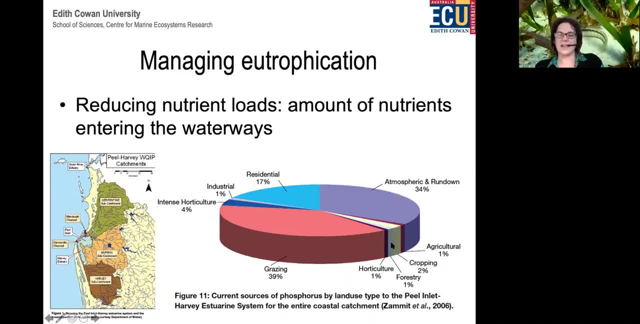 Only 1% comes from horticulture and 1% from forestry, and 1% from agriculture and 2% from cropping crops. So if you want to really focus on reducing the loads, then it's grazing and the residential areas where you need. 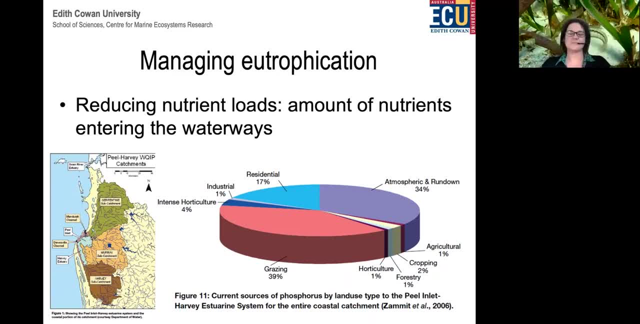 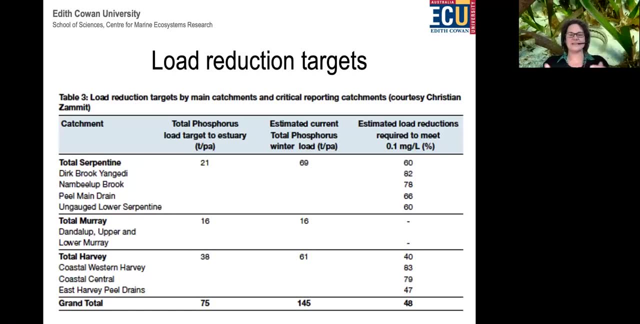 to put your most focus and effort in. So what a lot of the people do that work in this area is they do modelling. So they model the flow of the rivers and the groundwater coming into the estuary and they calculate, okay, how much. 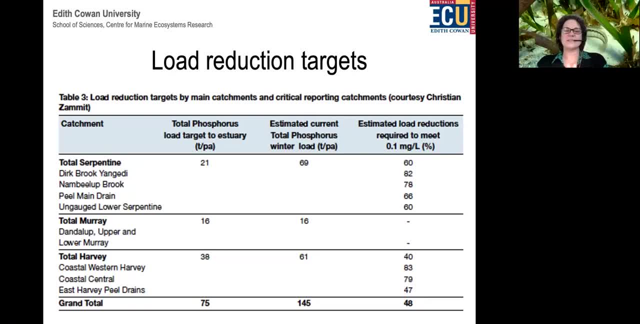 how many nutrients or what are the loads that are going to maintain a healthy ecosystem and stop it from sort of switching to the unhealthy eutrophic conditions? So in this case this table is showing the three main categories: The, the attachments, the serpentine, the murray and the Harvey. so they're the. 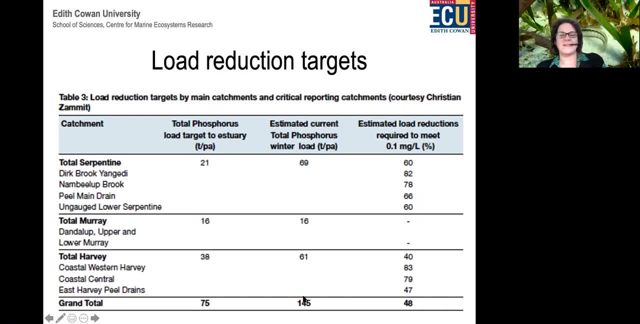 that's the column on the left-hand side. have a healthy ecosystem and then they work out exactly how much is coming in. so in this case, 69 tons per annum from the serpentine, 16 from the murray and 61 from the harvey. so you can see that. 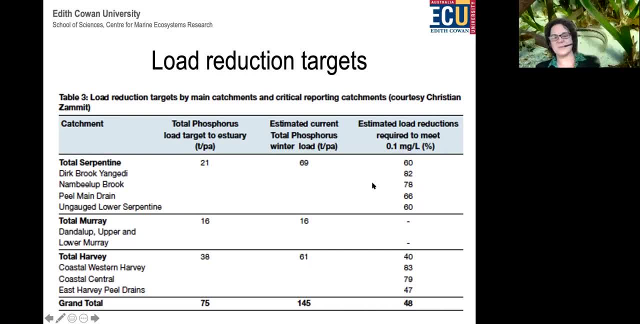 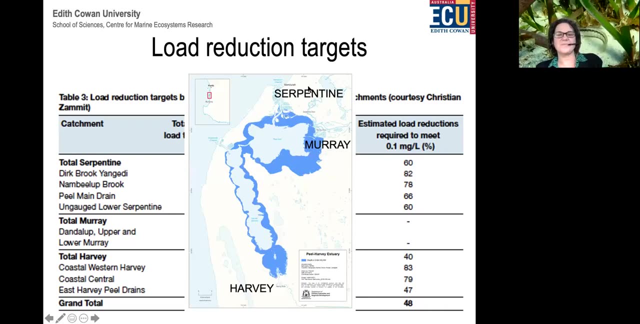 it's the serpentine river, which is in the very top of the catchment, and the harvey river, which is right at the bottom of the peel harvey. they're the ones where the most activity needs to be done to reduce those nutrient loads. so in this case it's the serpentine, up here, coming in sort of. 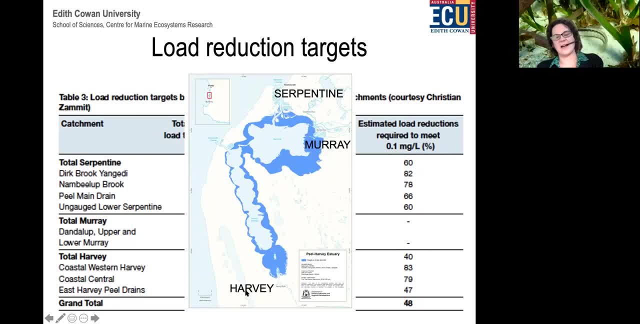 just to the east of mandra and the harvey river down the bottom, that needs to have the most action to reduce the nutrient loads. so those load reductions can be done through a variety of ways: through educating the, the farmers and the grazers, and the, the residential population, to reduce the, the nutrient use by planting. 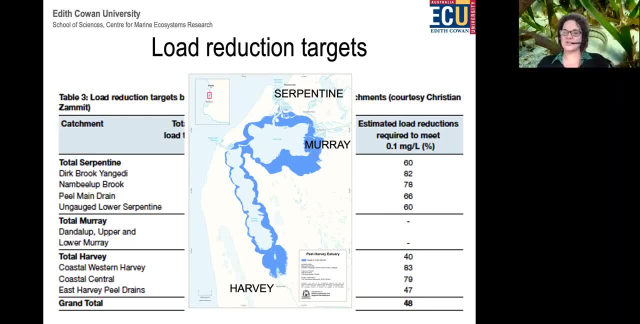 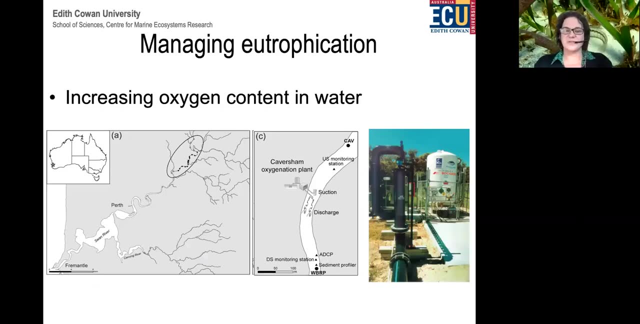 vegetation along the, the streams and rivers to take up the nutrients before it actually reaches the wetlands. so there's a variety of things that can be done in that space. so another way to manage eutrophication is by actually pumping oxygen into the water, waterways, and this is something that's done at a number of places, um in a in southwest um wa, so in. 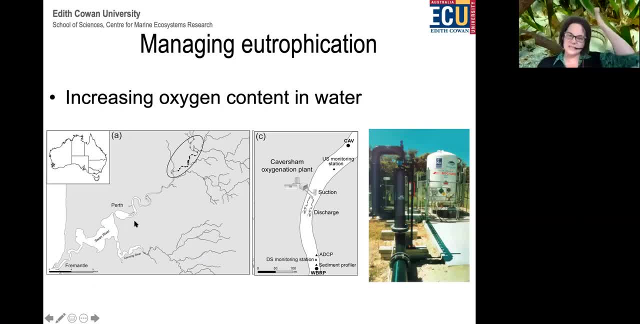 this case this is in the, the swan river or the swan river estuary. up near cabersham there's this oxygen plant and what happens? you can see where it says suction. the plant sucks water in from the river, pumps it through this oxygen um tank, which you can see, the picture on the right, and then 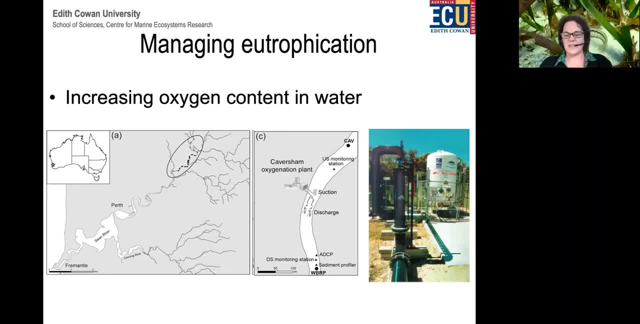 discharges it back out into the waterways, and this is something that's done at a number of places, and this is something that's done at a number of places into the, into the river, and this graph shows what happens when that system is turned on. so 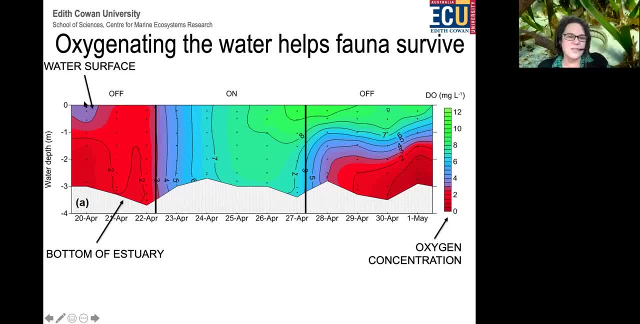 on the. this is sort of a graph: the top line is the surface of the water and the bottom line is the bottom of the river, and so the y-axis is the water depth and on the bottom is the dates. so this is looking at how oxygen changes over time and the colors. 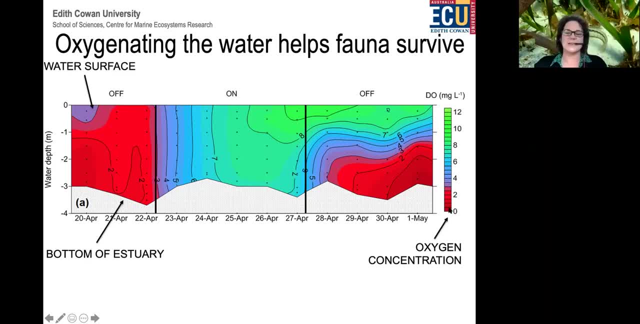 show you the oxygen concentration. so red is super low, blue is medium and green is a high oxygen concentration. so at this place in the swan river estuary, when that oxygen machine is off, you can see that there's hardly any oxygen there. it's red, so low oxygen. and then, on the 22nd of 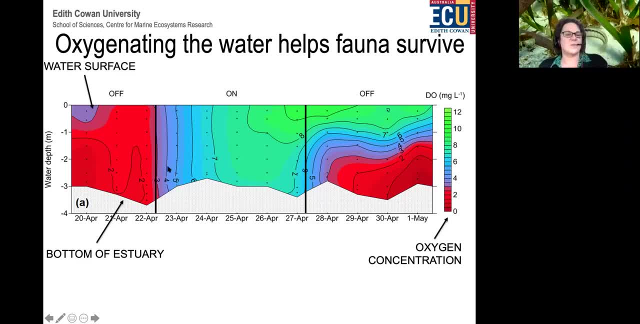 april, that machine's turned on and within 24 hours it's going from red to blue, showing that oxygen concentration is increasing, and then it's up to really high levels in a couple of days. then, on the 27th of april, that machine gets turned off and you can see. 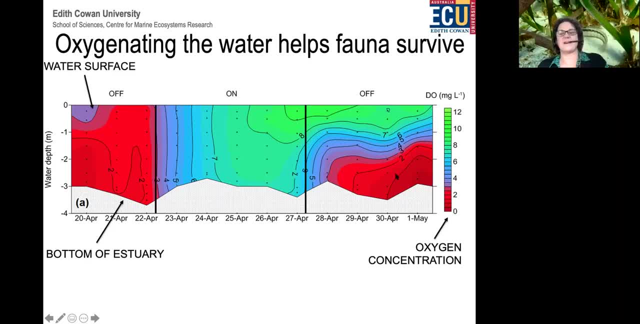 that oxygen concentration starts to get drawn down near the bottom of the river. it goes red again near the bottom, but there's still oxygen at the surface. so it can be really effective and quite rapidly, and this is really valuable. i think i've just my screens got stuck again. oh, here we go. um, because, if you think about it, fish. 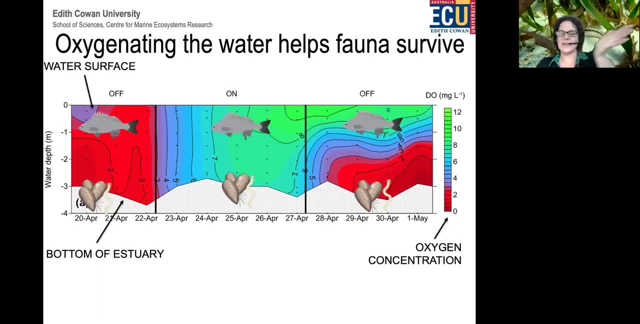 they can swim in the surface. if the oxygen gets low they can swim away and find some oxygen rich water. but the animals that usually live on the bottom, like the mussels and the worms- they can't really move very well, so they're likely to die when the oxygen concentrations are really low. 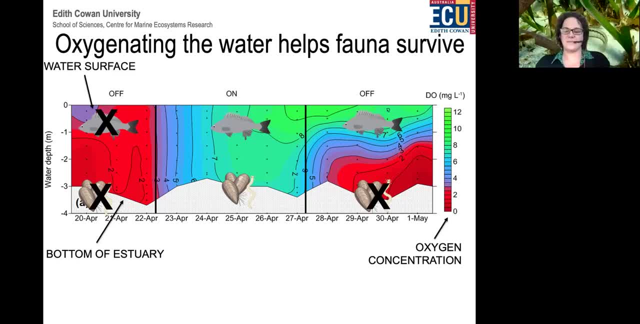 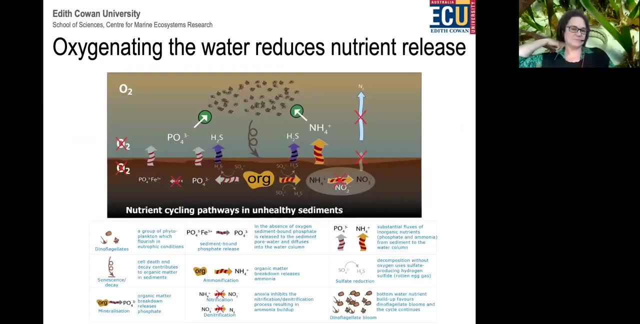 so there's real value in um helping the oxygen concentration and the oxygen concentration and the oxygen concentration and the support the biodiversity and the ecosystem by turning these oxygen systems on. but it's not only saving the fauna with these oxygen systems, it's also reducing the nutrient release from the sediment. so i said earlier on, when there's really low oxygen, 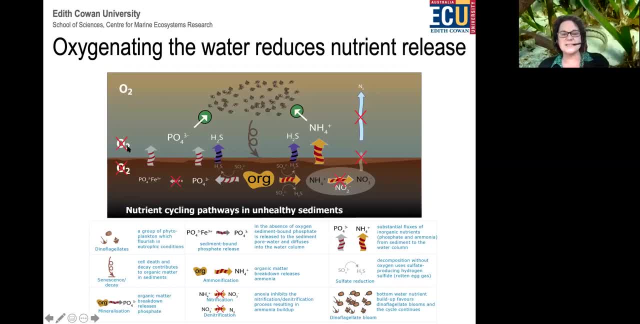 in the sediment or in the water just above, in the water column, just above the sediment. because of this organic matter breaking down, what happens is these low oxygen concentrations increase the rate of phosphorus getting released back into the water column, because phosphorus in with oxygen. it's usually 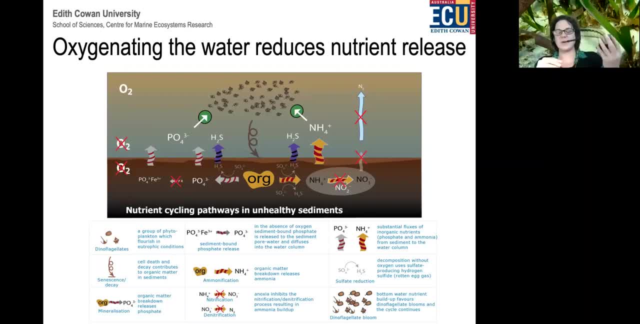 bound to particles but in low oxygen or no oxygen conditions it gets broken off from those particles and released into the water column. ammonium also gets released. so when you have low oxygen, these nutrients are getting released back into the water column and they get released back into the water column. 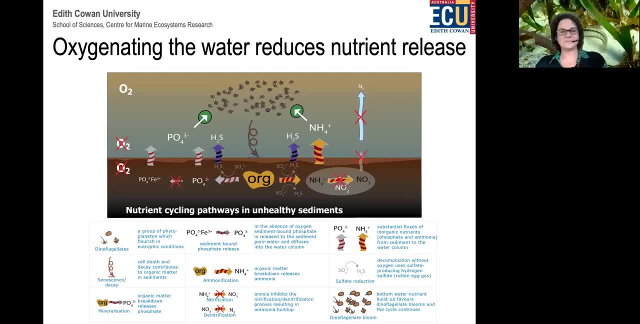 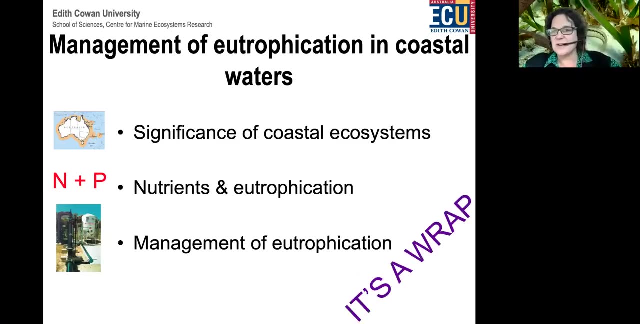 and they stimulate that phytoplankton growth again. so by adding oxygen it breaks that cycle and reduces the continual algal blooms. so that's, that's a wrap from me today about management of eutrophication in coastal waters. so i hope you've got a better understanding of why our coastal ecosystems are so important. 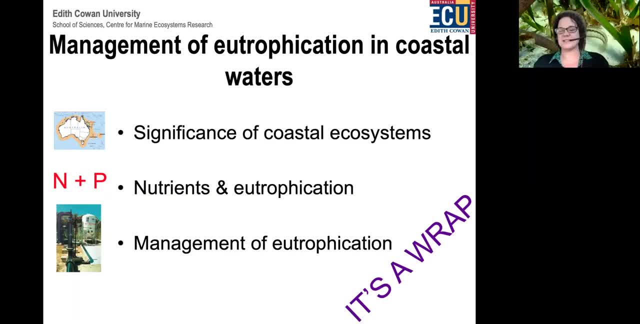 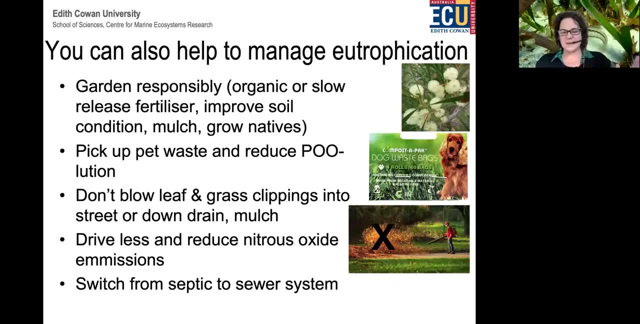 and how nutrients affect that process of eutrophication and how we can improve the eutrophication, and different management approaches that can be used- and it's usually these management processes that i talked about- have been activities that are managed by government or industry, but you also can make a difference to managing eutrophication. 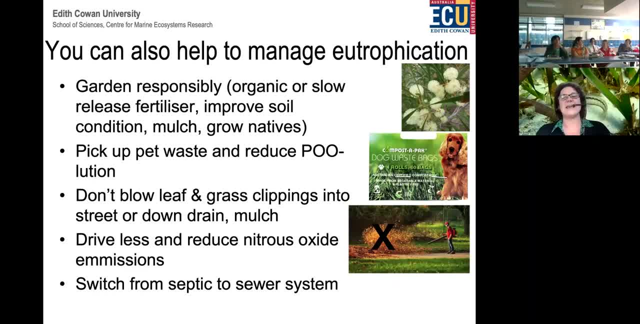 and reducing the nutrients that are getting to our waterways. if you like gardening, certainly think about using slow release fertilizers or using organic nutrients that are getting to our waterways, if you like, organic mulches to improve your soil condition and grow native, so you don't. 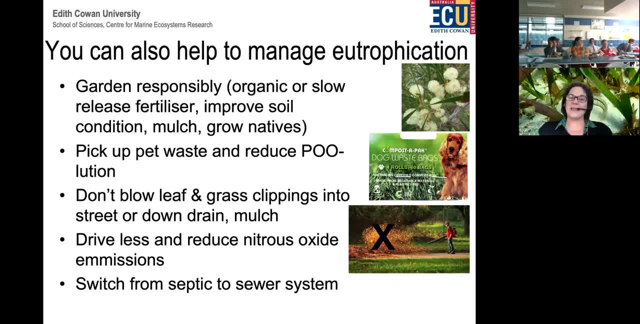 need to add as many nutrients, pick up any pet waste and reduce that pollution, so that all the the waste from your pet isn't getting washed into the waterways and the storm drains. you can make sure that you don't put leaf and grass clippings into the street or down the drain, because that 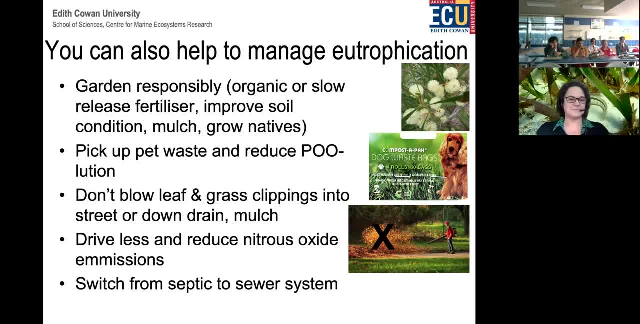 increases the organic matter reaching our waterways. driving less is going to reduce the amount of oxide emissions and that atmospheric deposition that occurs. and, if you can, if your property is still on septic and you have the opportunity to switch to a sewer system, that's much better. 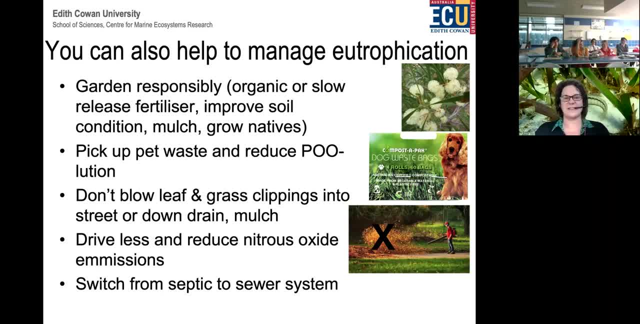 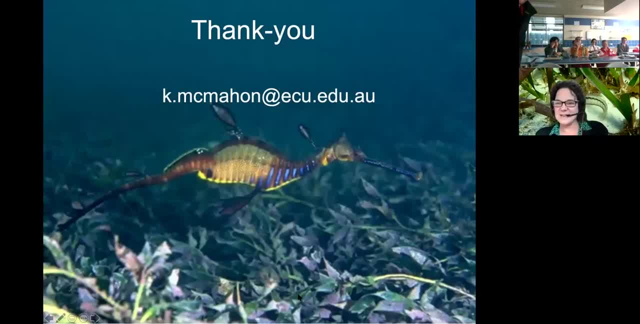 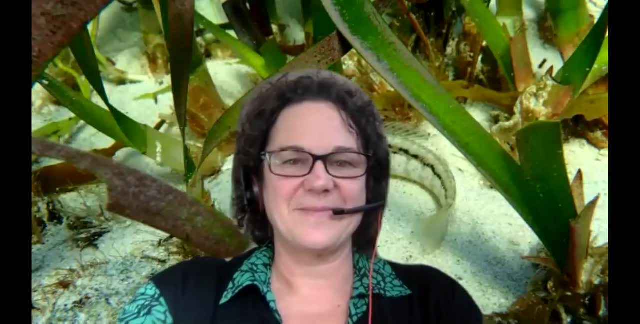 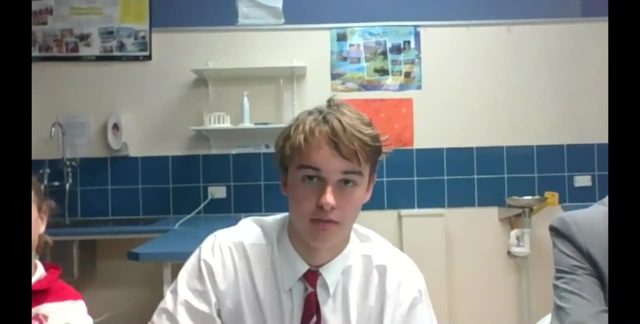 because the nutrients can get taken out much more effectively in that kind of system. so that's all from me. thank you very much. has anyone got any questions? and i've got a few minutes left. um, how often do you see eutrophication in perth, and is there like a time of year where 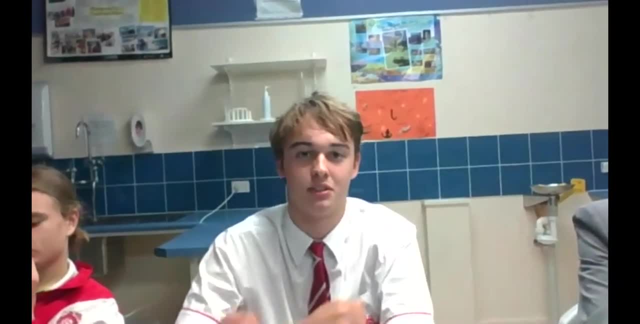 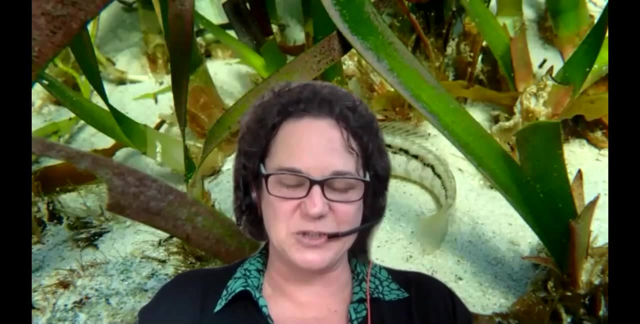 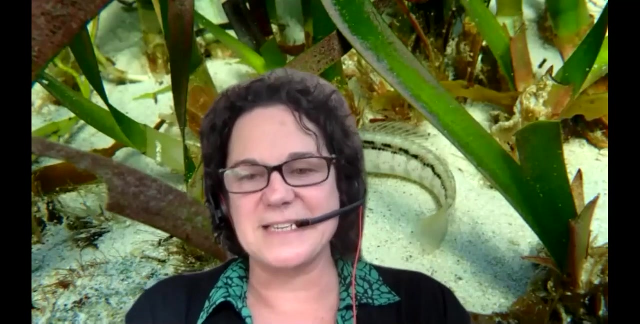 it's like in most common and like it increases. so once a system is going through eutrophication, it's it's eutrophied. so the swan river estuary is eutrophied um less than all the vast one are up. but there are particular times when you're much. 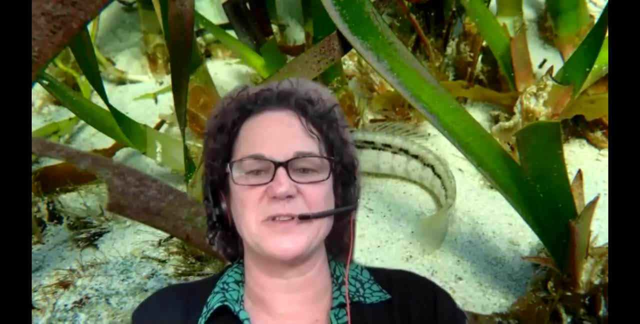 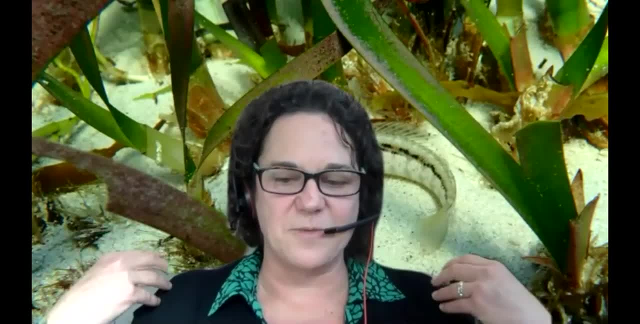 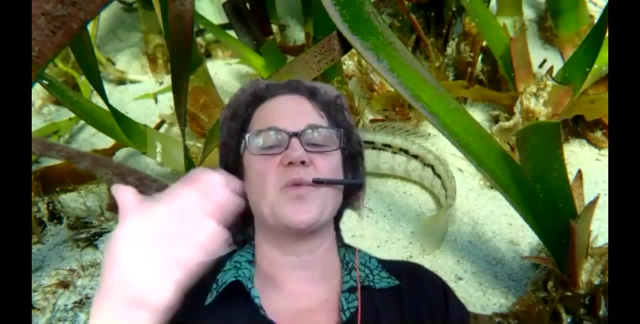 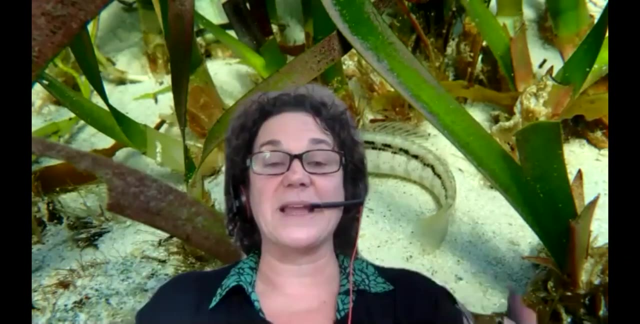 after the winter rains, because when it rains the washes the nutrients from the catchment into the river, and then, after the winter rains, in spring we're getting warmer temperatures, so that increases the rate of phytoplankton growth and also, if you've got really calm conditions. 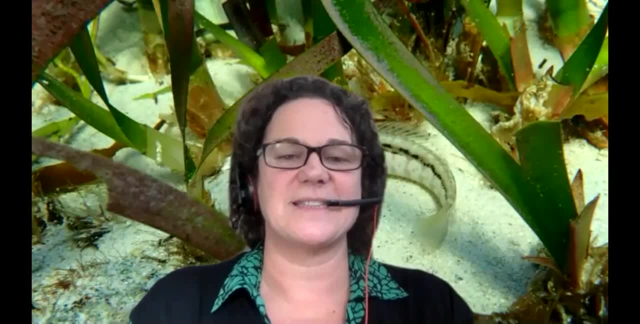 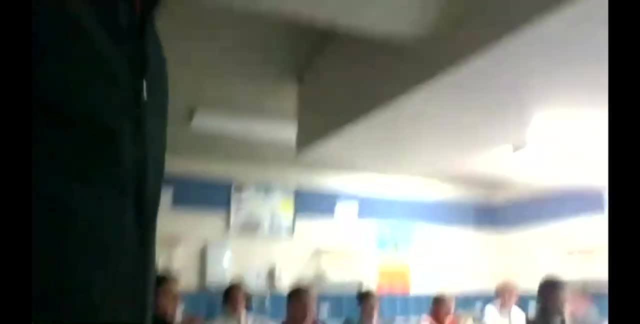 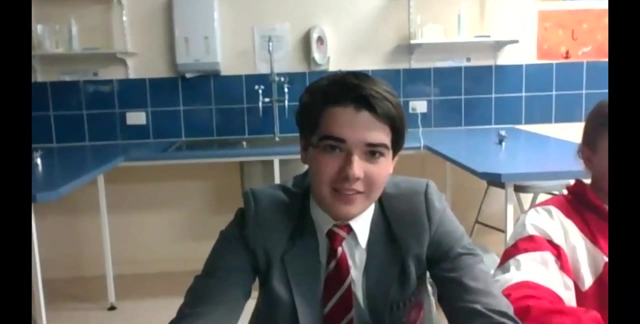 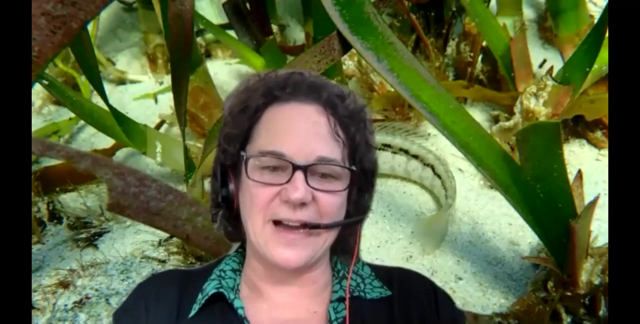 they are the sort of the three key factors that are likely to result in a phytoplankton bloom. um, in the experiment, how did you measure the amount of plankton in the beaker? well, i actually didn't do that experiment, but i have done them and there are a number of ways. 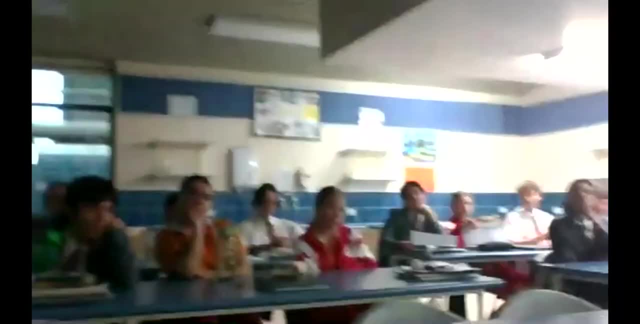 that you can do it. um, so you can take samples over time and count under a microscope the number of phytoplankton blooms, and you can do that by counting the number of phytoplankton in the beaker. and you can do that by counting the number of phytoplankton in the beaker.